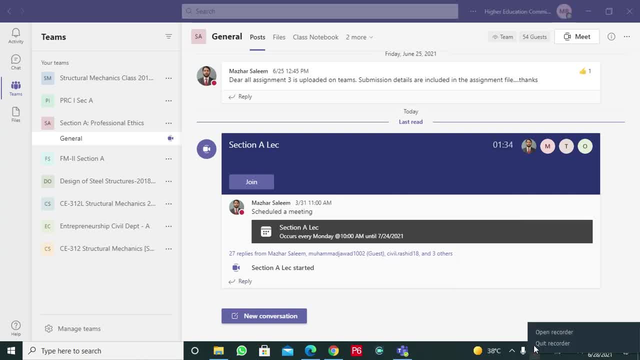 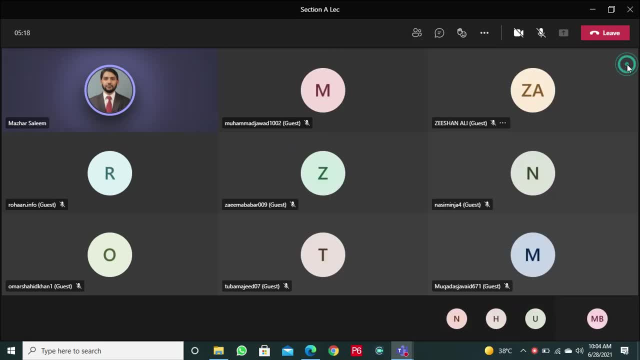 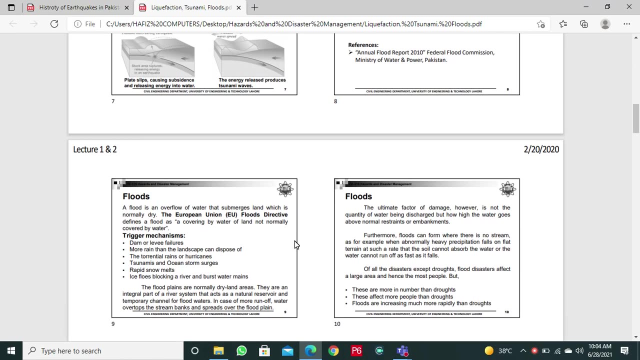 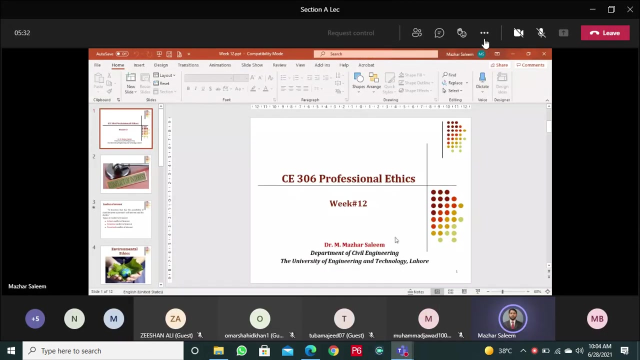 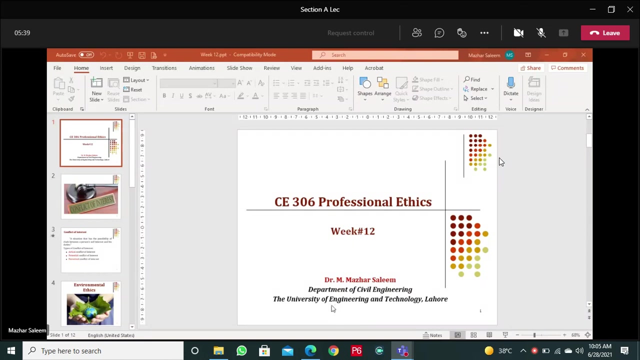 Let's start our discussion. Let me share my screen with you guys. Okay, Can everybody see the PowerPoint? Anybody please come forward. Can you guys see the PowerPoint on your screens now? Jabbat Bilal. Okay, Thank you. 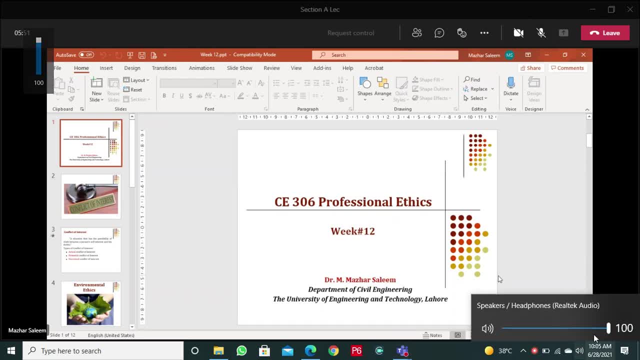 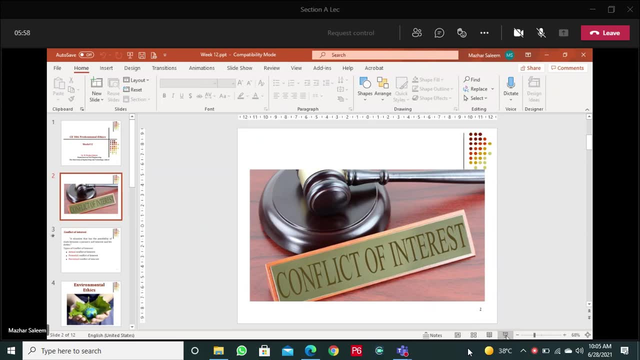 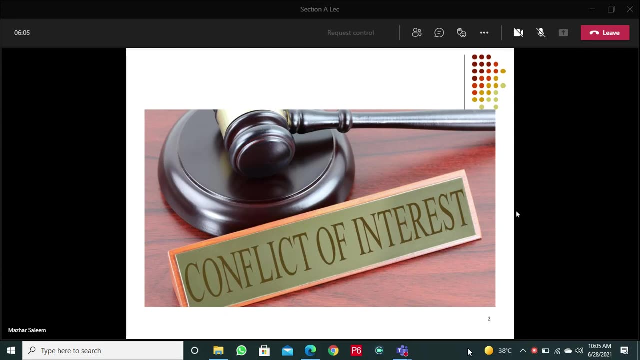 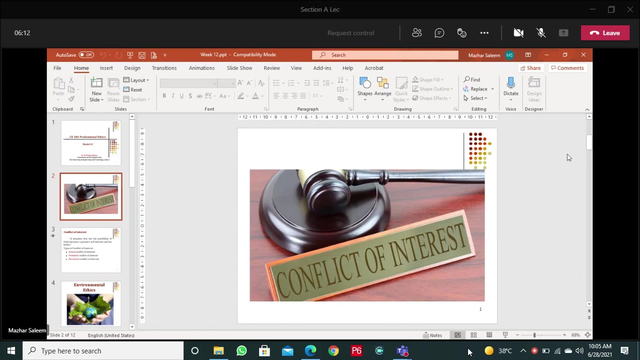 Alright, So let's start our discussion. The first topic that we are going to talk about today is about conflict of interest, And I think we have We have discussed conflict of interest before as well, So before I explain it to you, I would like to hear some points related to conflict of interest from you guys. 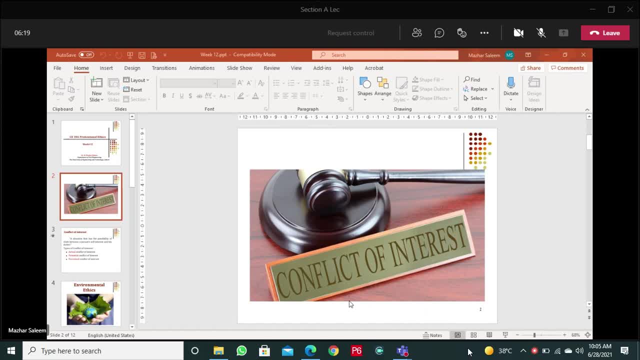 So can anybody comment on this? What do you mean by conflict of interest? Any volunteer? Look at this. Look at this. Are you there? Look at this. Javit Look at this. Looks like she is not there, Nasir. 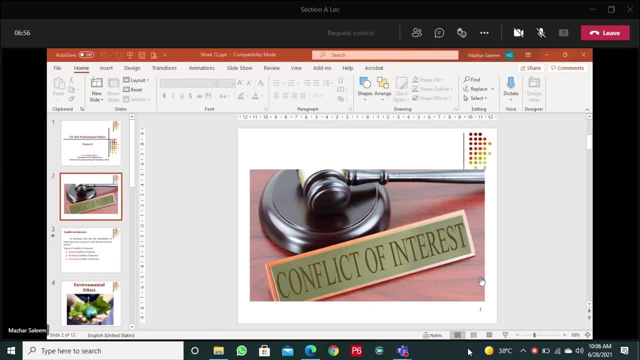 Nasir, Yes, sir. So, Nasir, what do you know about conflict of interest? What is conflict of interest? We have talked about that before, Sir. conflict of interest can be developed in such a way that the interests of the person you are working for and the organization you are working for are not matching with your own interests. 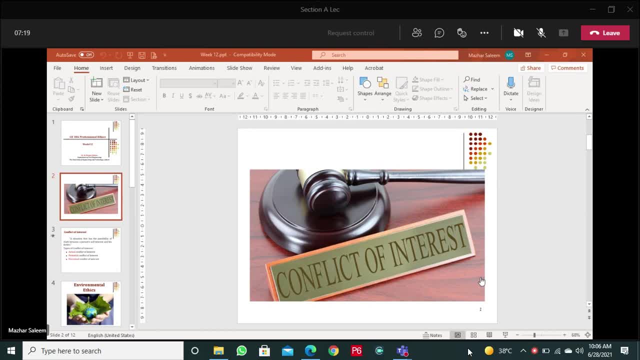 And you prefer to give your own interests and give your own personal interests. Conflict of interest can be a client or a contractor who doesn't want to sell his money and doesn't want to give him the best product. However, a contractor wants to make maximum profit. 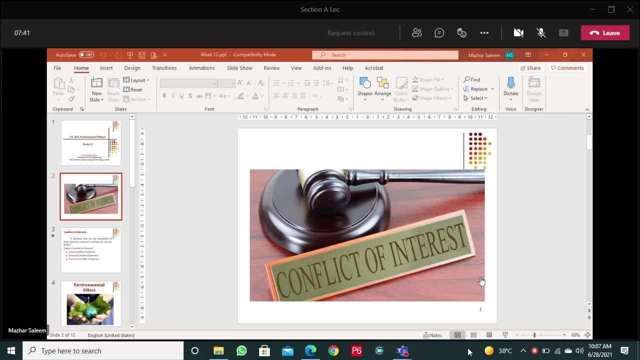 Hence you call it conflict of interest. Actually, this conflict of interest is defined for one person or for one organization, Whenever there is conflict between two organizations or two individuals, that is. we don't call that as conflict of interest, That is just a general conflict. 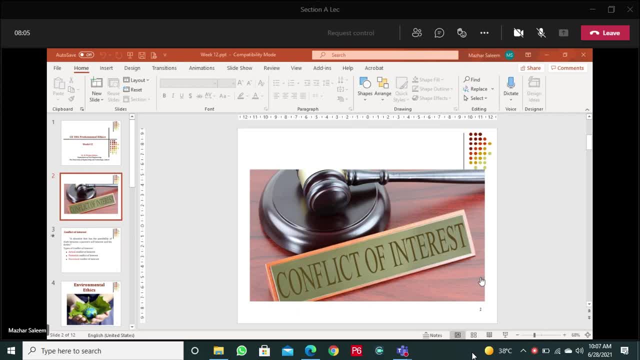 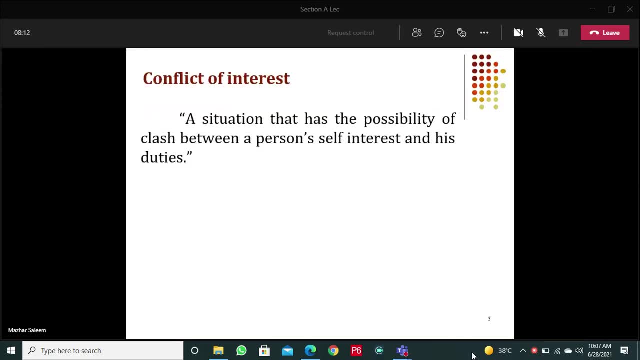 So conflict of interest is basically a problem. Conflict of interest is basically a problem. Conflict of interest is basically a problem- one individual or about one organization. Let's see how do we define it formally? So a situation that has the possibility of clash between a person's self-interest and his duties. 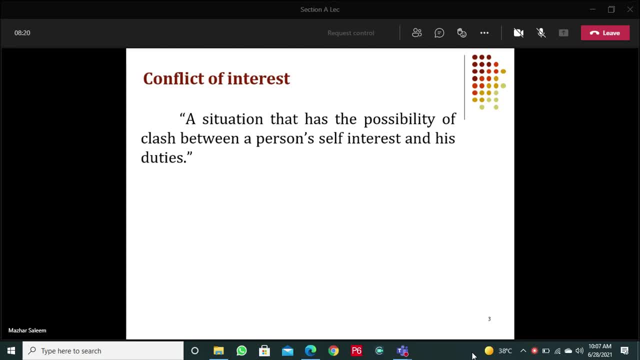 So if there is a conflict of interest between an individual's personal interest and his duties, then we call it conflict of interest. And conflict of interest occurs in probably all fields. It's not just a phenomena which is limited to civil engineering. In every field or in every person's. 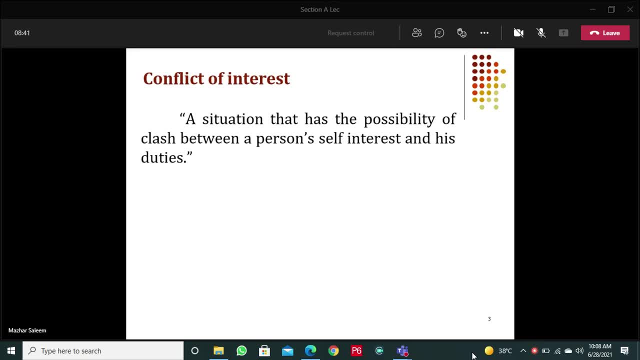 life, there is a conflict of interest experienced at some stage. There are many common examples of this in the civil engineering perspective, For example, if you are, let's say, a structural designer- I think we have discussed this example before as well, that you are a structural designer- 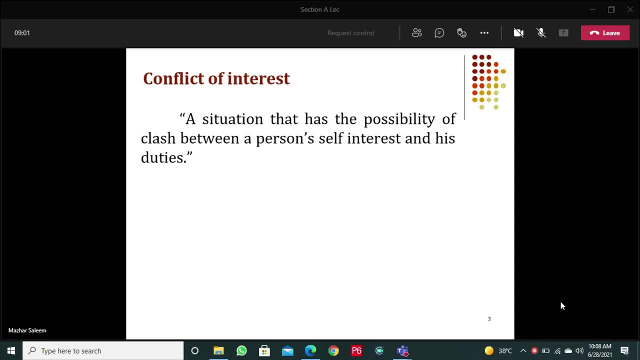 and you work for a company that provides structural design services. Now, once you have gained certain experience and learned certain skills, you might think about starting your own consultancy services. So, in parallel to your job working in that organization, you start your own consultancy services. Now, if any client comes to that organization. 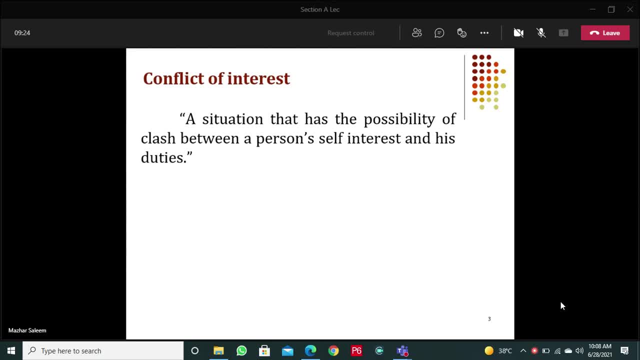 the organization's interest is that the client sticks to that organization and gets services. then the company can make money. But your personal interest would be that the client should take personal services from you. then you can make more money because your salary is fixed If the client is taking services from you as an individual or as an 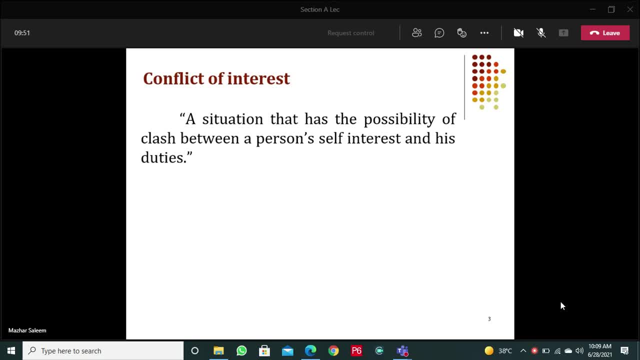 independent consultant, then the fee will come to your pocket. So in this situation we will say that there is a conflict of interest. And another example of conflict of interest in, for example, if you have a client who is an individual or as an independent consultant. 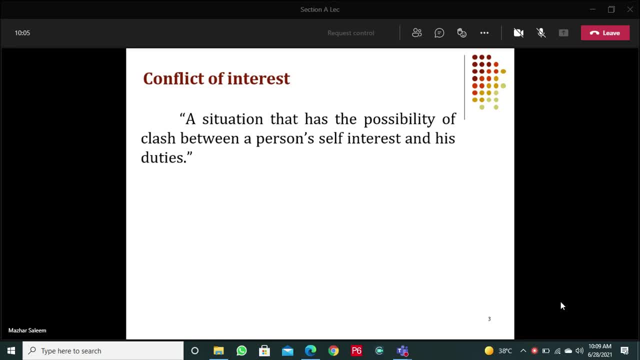 you can make more money because your salary is fixed. If the client is taking services from a company and from the contractor side is that, let us say, you are in charge of a site and you are also responsible for procurement of material. Now, if you have 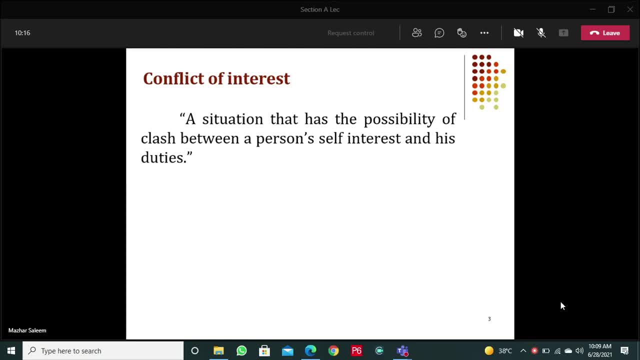 connection with certain vendors who would like: oh, You are getting commission from certain vendors. you would like to buy material from those vendors, regardless of the quality of the materialSo in this situation, we will say that there is a conflict of interest. 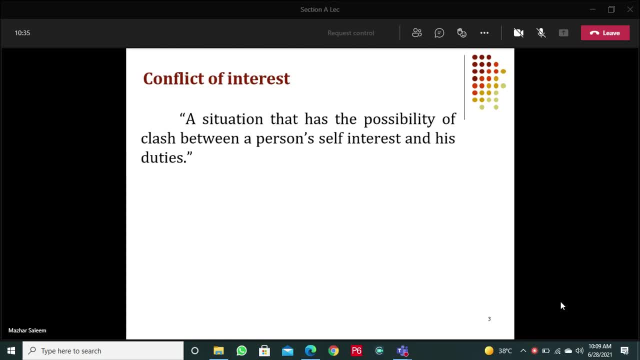 conflict of interest in your personal. so there is conflict of interest in your like, in your personal interest and in your in your duties. so you might think about compromising on the quality of the quality of the material just to make more money. okay, so these were a couple. 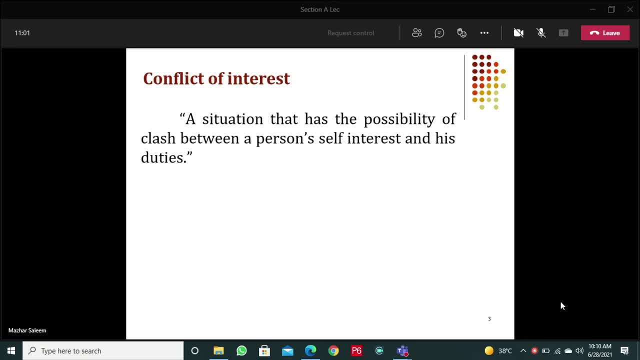 of examples from from civil engineering perspective and if we think outside of the civil engineering, as i said, that almost in every field we see conflict of interest. now one of the example maybe. let's say there is a judge in the court of law and now if a judge is hearing a case? 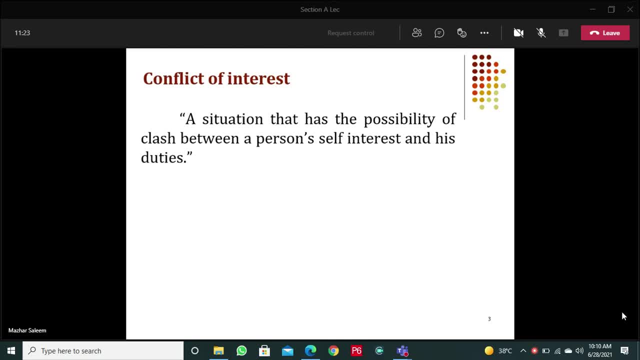 of his friend or his relative or his family member. now that judge most likely will have bias towards that family member or that friend. now his duties as a judge is to is to provide justice, disregard of anything right. but if he's hearing a case of a closed one then he might have a bias. 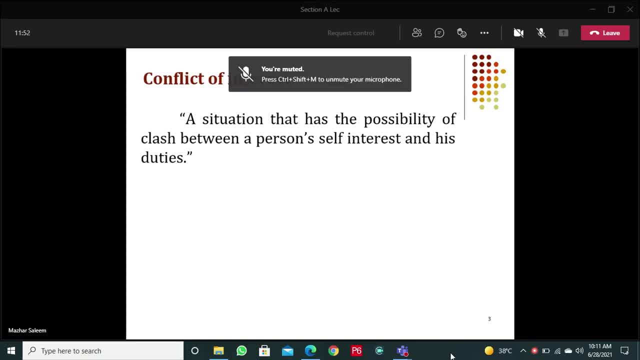 towards that that person. so this is another example of conflict of interest. okay, now there are a few types of conflict of interest as well. one is the actual conflict of interest. when the conflict of interest actually exists and you are pursuing your own benefit, or you are you are giving priority to your own interest as compared to your duties, you will say that conflict. 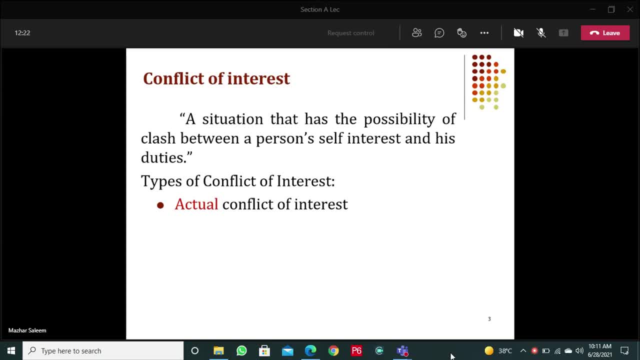 of interest actually exists. that is termed as actual conflict of interest. what is potential conflict of interest? potential conflict of interest is when there are chances that you may exploit the situation for your personal interest. now you may or may not be doing that, but there are chances that you may. 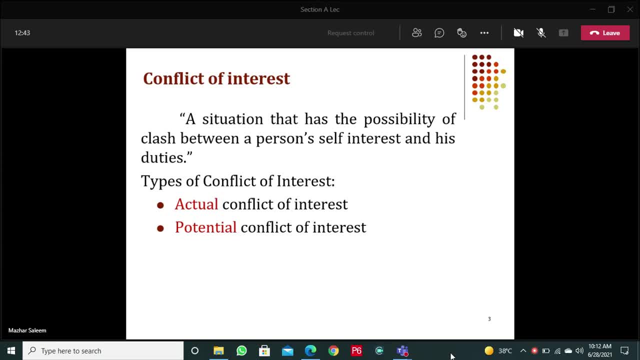 exploit the situation. so such situation is done as a potential conflict of interest, and the third type is known as perceived conflict of interest. now, what do you mean by perceived? perceived conflict of interest means that there is a perception that conflict exists between your personal interest and your duties. in reality, that 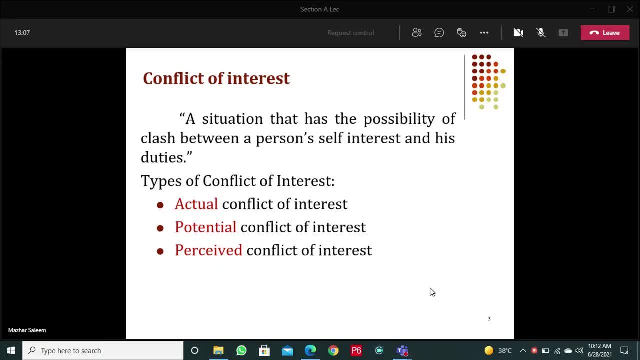 you might not be pursuing your self-interest. you might be fulfilling your duties, but under certain cases- for example the case of the judge that the example that i gave- the perception might exist that you are benefiting one of the parties. so when such perception exists, we call that as perceived. 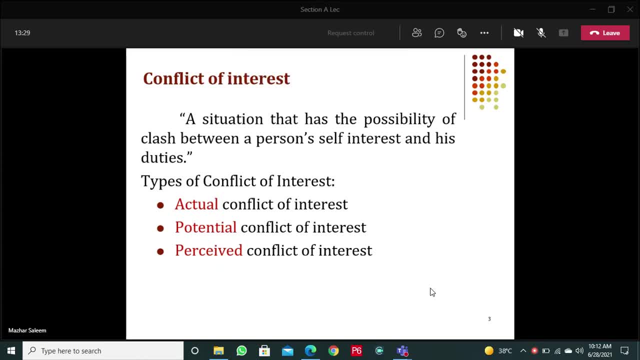 conflict of interest and, as a responsible professional, it is our responsibility to avoid conflict of interest in whatever form it exists. and one good ethical practice is that wherever conflict of interest exists, you clearly state that conflict of interest and you remove yourself from from that situation. that is the ideal way of dealing with conflict of interest. 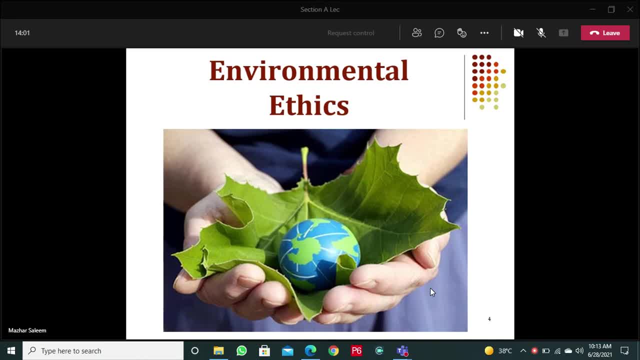 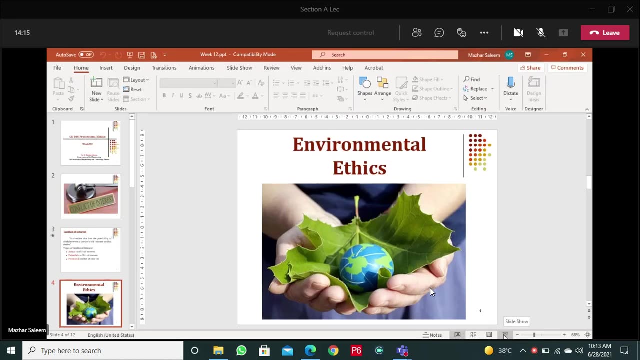 right. so this was the first topic that we wanted to discuss today. now let's move to our next topic, which is environmental ethics. but before that, i would give you a chance to ask any questions, if you have any questions about conflict of interest, and in addition to that, i would also like somebody to comment on environmental ethics. 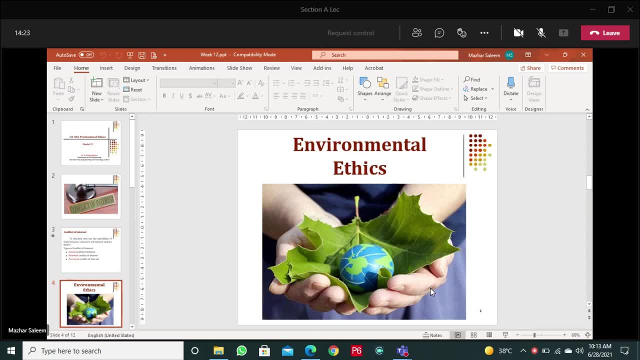 what do we mean by environmental ethics and what are our responsibilities towards environment? okay, i see somebody has raised his hand, yes, sir, so my question is bit of interest, definitely, so my question is: maybe a public services provided there, there, so what about that? what will happen so? 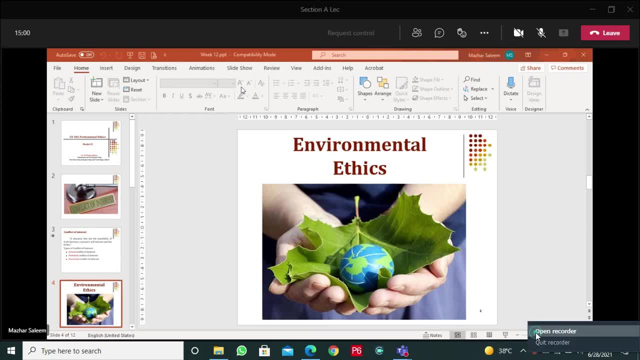 if you have a job in a company. it only arises when you are doing a job in that company, which is, let's say, a structural design and provides any services, and in parallel you are providing your services, and in that too, the real problem is when you are actually channelizing your clients towards you. 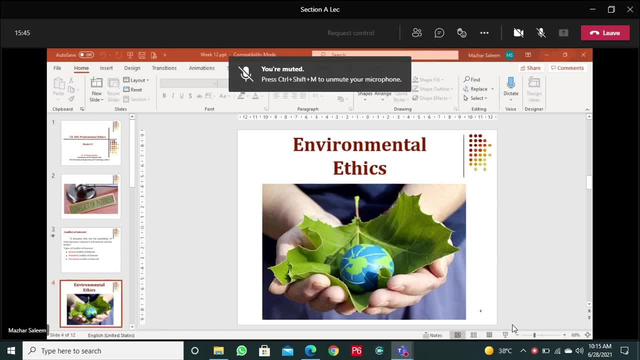 if you are doing a job in that company and while doing a job, the client of that company, you are channelizing your clients towards you. you have, you are serving it, when the other manus in terms of work into that company, you are small, you are only impersonating a kind of employee. 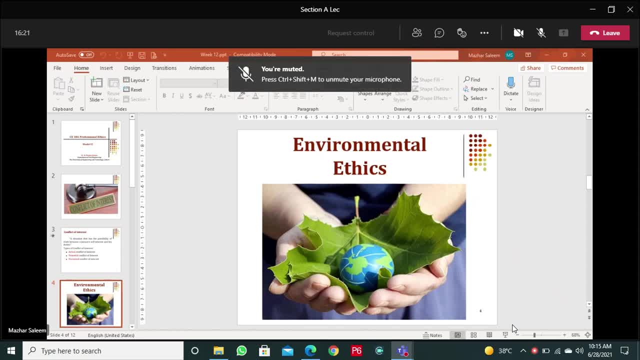 and now in contracts. If you are providing services in parallel, then we will not call it a conflict of interest. It is totally fine. If we don't maintain a certain kind of contract, then it's fine. If you leave the company and carry on working after that, it's totally fine. 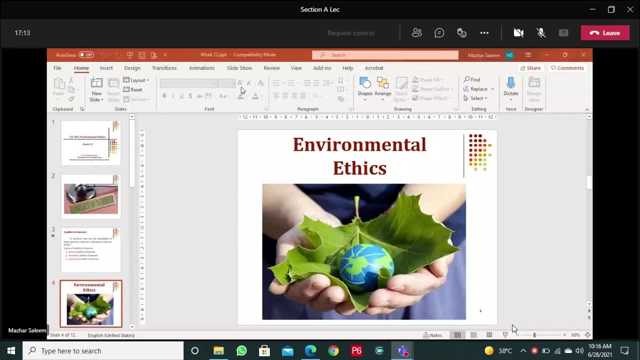 In parallel, You can provide services, but you have to make sure that you don't take it away from the company, And the services that you provide as a freelancer can also be provided by the company. What are environmental ethics? It may be about highlighting the importance of environmental values. 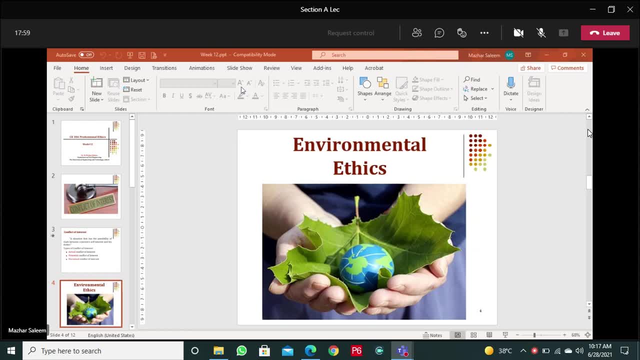 And raising awareness For its protection. in simple words, What can be an example of this? How is the environment affected And what can be done for it? First of all, we see it on a daily basis: Global warming, This and that. 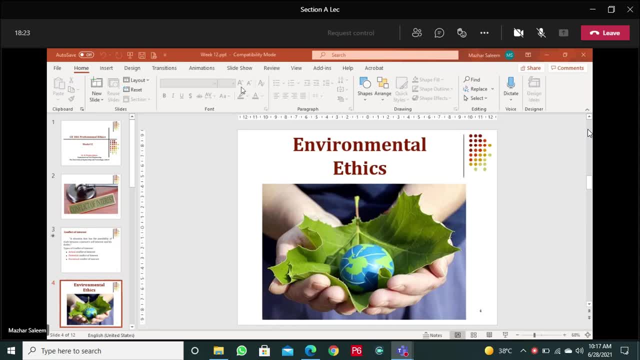 For its preservation. our government has taken a step: Billion trees, tsunami- To pull down Pakistan to a bit. Sir, I guess this is how it happens. There are a lot of issues. These are not only at the country level, They are also in the UN. 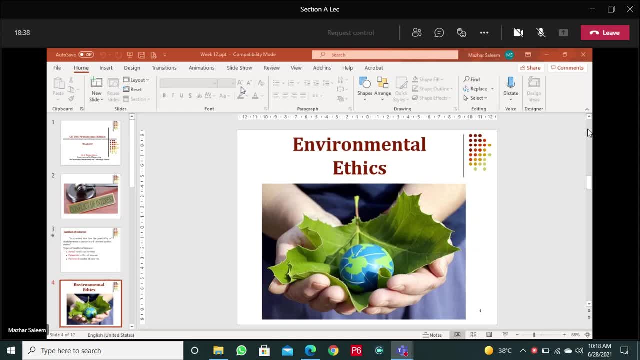 But, sir, I don't think it is as important as it deserves. Alright, Like you said about the Billion Trees Tsunami, This was initiated for environmental protection, So environmental ethics specifically talk about our responsibilities towards the environment And how we are supposed to treat the environment. 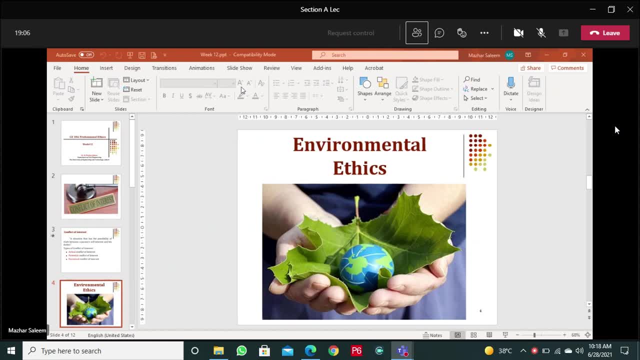 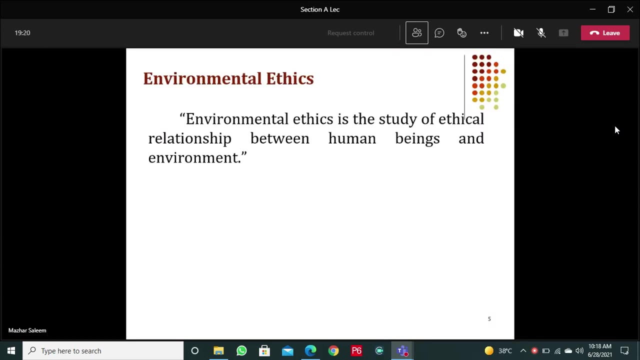 And how we are to perform our activities So that we can minimize the harm to the environment. Let's see how do we define it And what are the factors that are important in this regard. Environmental ethics is the study of ethical relationship between human beings and environment. 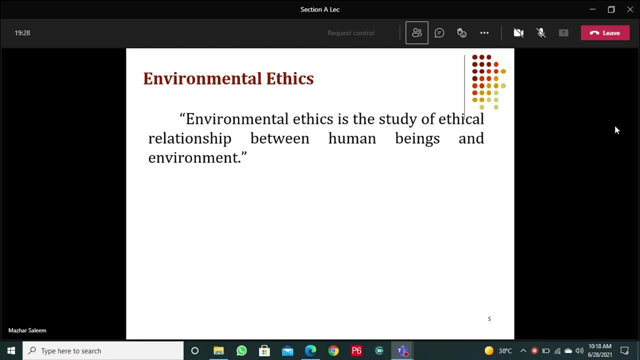 So, as a human being Like it, is our responsibility to take care of the environment, And our relationship with the environment is termed as the environmental ethics, And environmental ethics provides basis for the fields of environmental protection, Animal protection and nature protection. So these three further fields are based on environmental ethics. 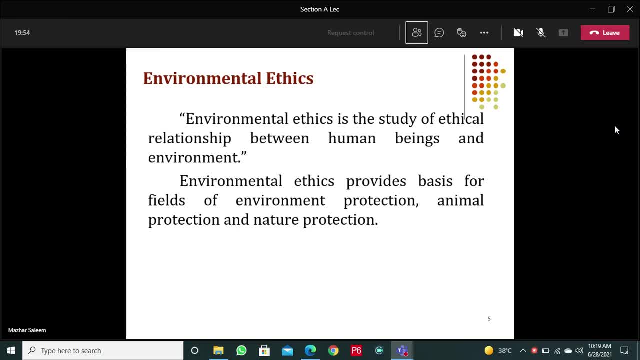 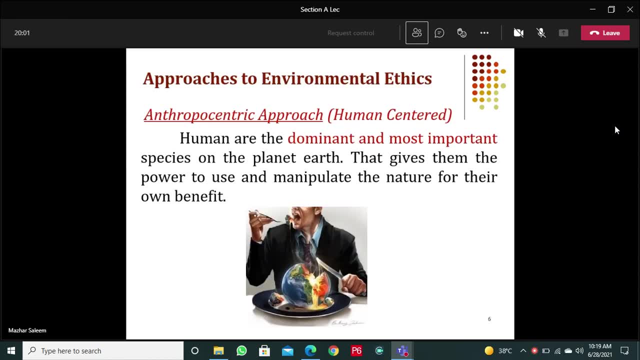 When we study environmental ethics, Then these are the three further branches: Environmental protection And nature protection. Now there are two different approaches worldwide for environmental ethics. First approach is termed as anthropocentric approach Or human centered approach, And this approach says that the human beings are the dominant and most important species on the earth planet. 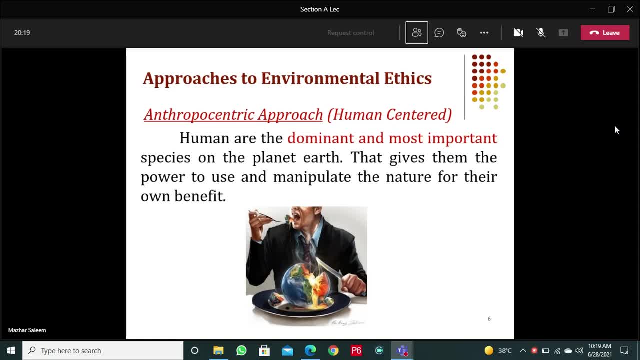 Okay- On the planet earth And this gives them the power to use and manipulate the nature for their own benefit. Okay, So whatever human beings think that is needed for them, Whatever is required for the good of human beings, Human beings can do that. 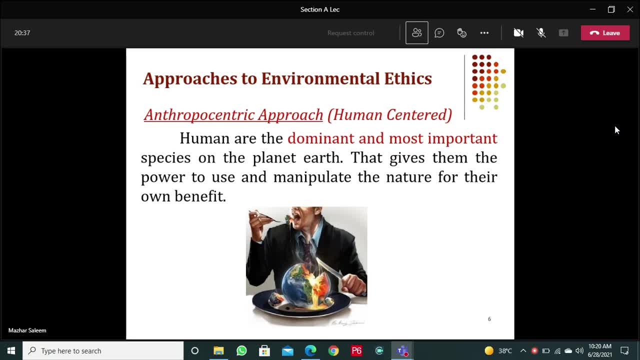 And environment or everything else is secondary. So this image It well describes this concept of human centered approach: That the human being is supreme And the human being can use all resources to fulfill his needs. So this approach is known as anthropocentric. 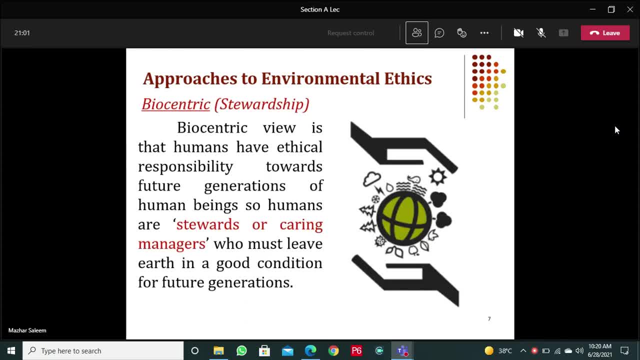 Or human centered approach. And then there is another approach, The second approach, That is biocentric approach Or stewardship. Biocentric view is that human beings have an ethical responsibility towards future generations of human beings. So humans are stewards. 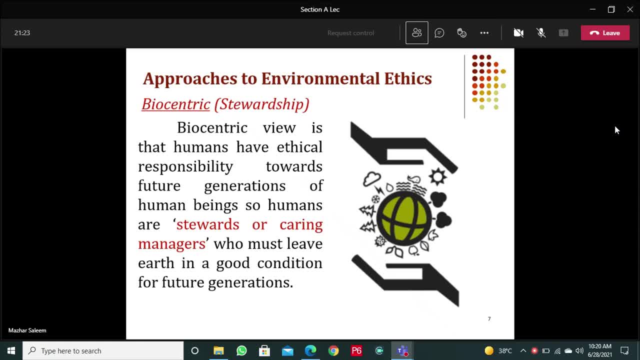 Who must leave earth in a good condition for future generations. So as a human being, According to biocentric approach, We have a responsibility to take care of the environment. It is not that we are the most important species on the planet, Or probably we can still say that we are the most important. 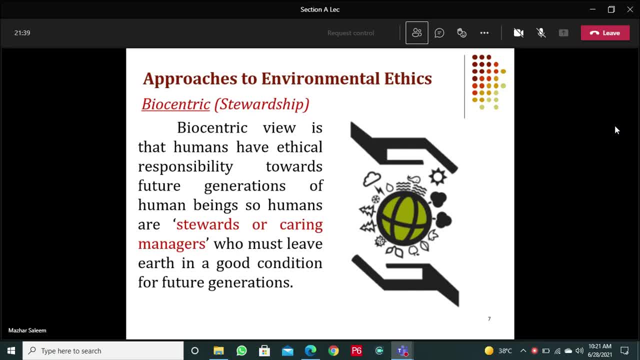 But still, we need to take care of the environment, Not only for our coming generations, But for the other species living on the planet as well. Okay, If we are doing a lot of deforestation Or we are Contaminating the water bodies. 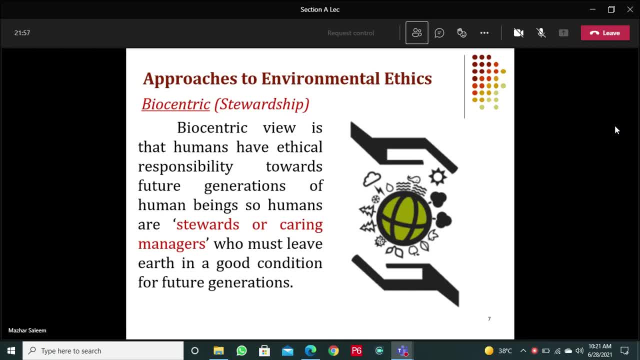 We are contaminating the air, So this is not only harmful for our next generations, Or even for our generations, But it is also harmful for the other species living on the earth. If you are polluting the water, Then all the sea creatures. 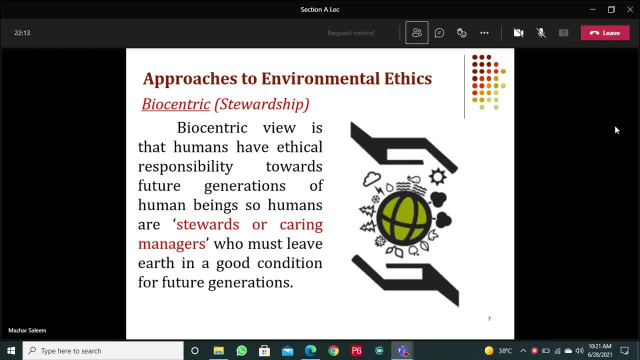 Or water creatures. Those will get negatively affected. Similarly, if you are polluting the air, Then all other creatures Who breathe in air Will get polluted. So you can see that If we are creating noise pollution, That will affect all the species. 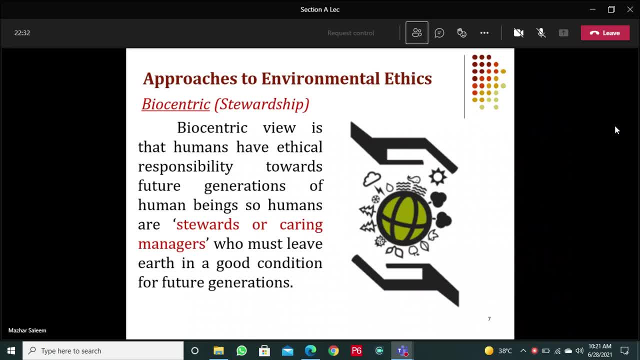 On the earth. So in biocentric approach. This approach says that We have the responsibility To take care of the entire planet As a human being. Okay, And this is why we are called as stewards. And this biocentric approach. 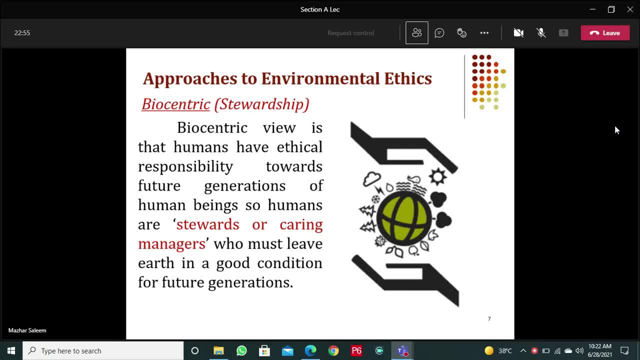 Is actually The basis of Sustainable development. We have talked about Sustainable development before, So this biocentric approach Provides basis for the sustainable development. Now, when we talked about Sustainable development earlier, I gave you a few examples That how civil engineers are contributing. 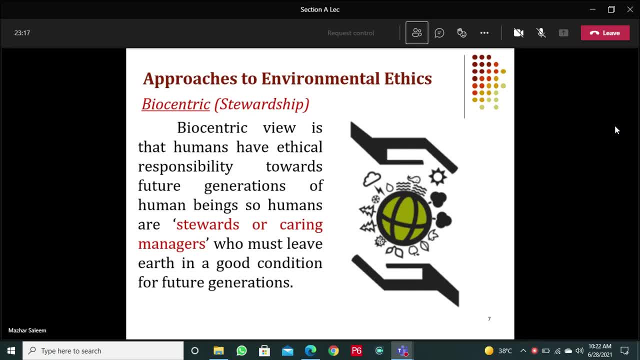 Towards sustainable development, And I can quickly Repeat those examples here. One example is When we Demolish concrete structures, A lot of Waste concrete is segregated And utilizing that waste concrete Or disposal of that waste concrete Is a problem. 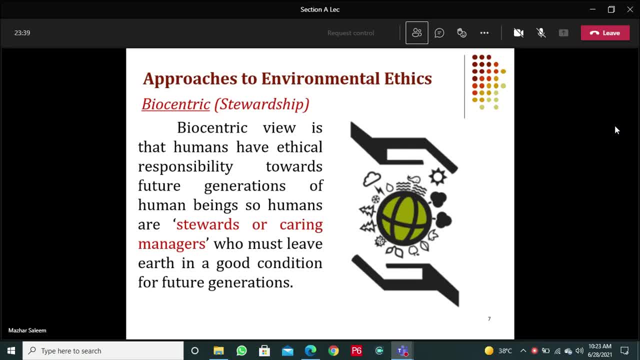 So what we are trying to do currently is That we are trying to recycle that concrete And get aggregate from that concrete And use that for For newer concrete And there are Specific uses of that concrete. So Use of recycled aggregate. 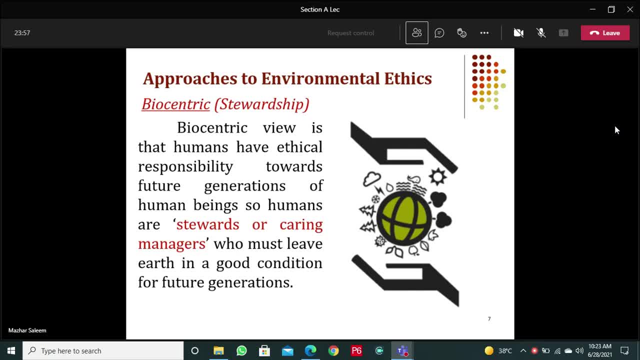 Not only helps us in In Appropriately disposing Of the waste concrete. Further it helps in In a reduction in Resource depletion, Because we are consuming large quantities of aggregates, But if we are Recycling those aggregates, That will decrease the resource depletion. 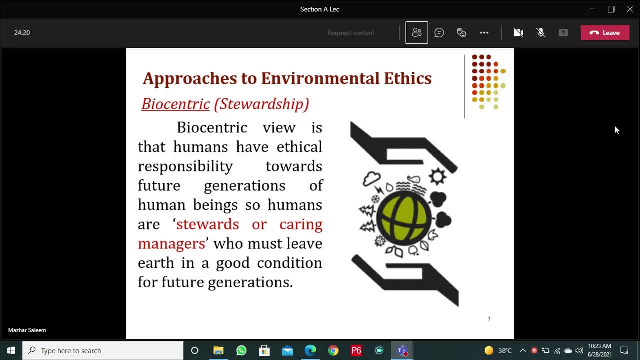 So this is one example. Second example is that we are trying to add Other waste, Like waste marble powder Or waste fly ash, Into concrete as a Cosmetic material And, as a result, It contributes to the strength of concrete, Concrete strength. 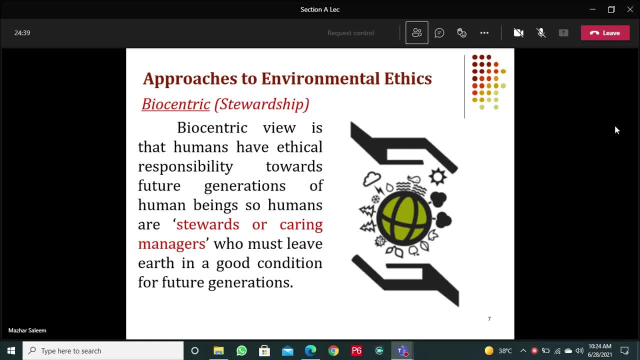 And that causes A reduction in the demand of cement. So Then production of cement will also be decreased, And that will help the environment, Because production of cement generates Carbon dioxide. So Cement is decreased, Production of cement will be decreased. 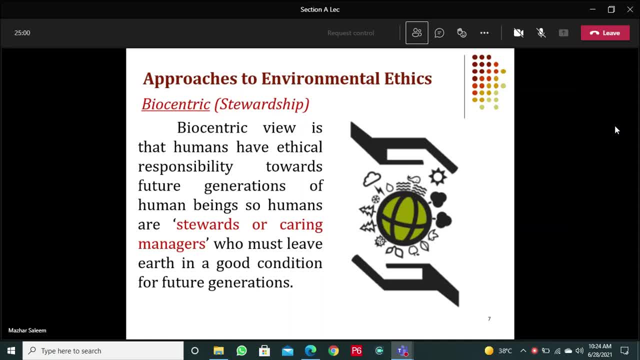 And the environment will remain clean And, similarly, We Like. there is another Another advantage of it is that We will be using some waste material Whose disposable was an issue Before. So the waste material Who effectively used. Another example of the contribution. 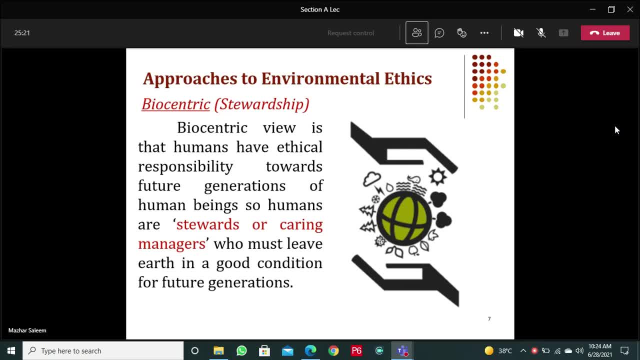 Of civil engineers To concrete. That is a very new concept In our part of the world Internationally. Our department has recently Initiated research on that. One of our students is working on that. That we are trying to add. 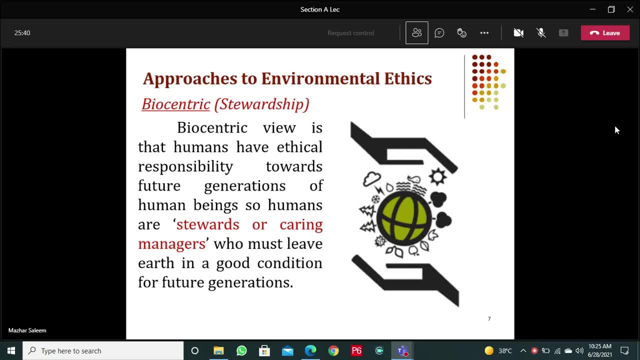 Carbon dioxide in the concrete While mixing the concrete. That helps in Removal of carbon dioxide from the environment. Further, it contributes To the strength of concrete as well To carbon dioxide That causes. That increases the strength of concrete And, as a result, 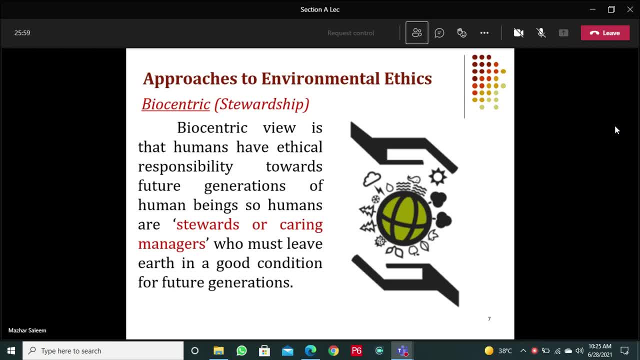 We have to use less amount of cement To gain same strength. So this is another way in which We civil engineers are contributing Towards Sustainable development. So the concept of sustainable development Comes from Biocentric approach. The pollution. 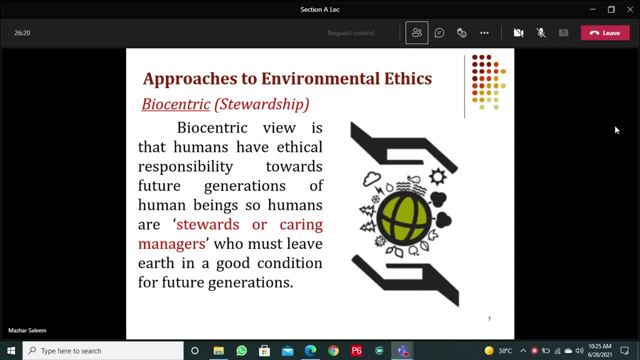 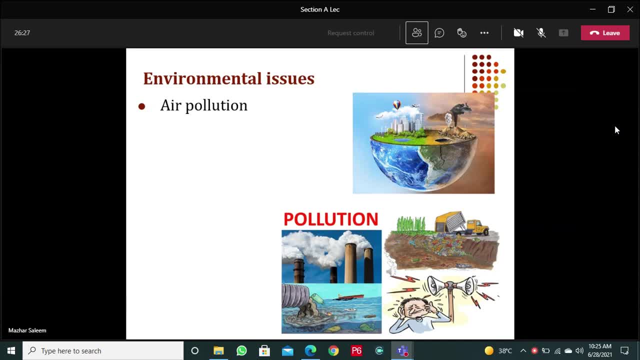 We cause in the environment As a Sustainable In general. Let us see what are different sources of that Air pollution. All the industry Creates air pollution. Government has made laws on that. How much contamination you can, What level of contamination you can. 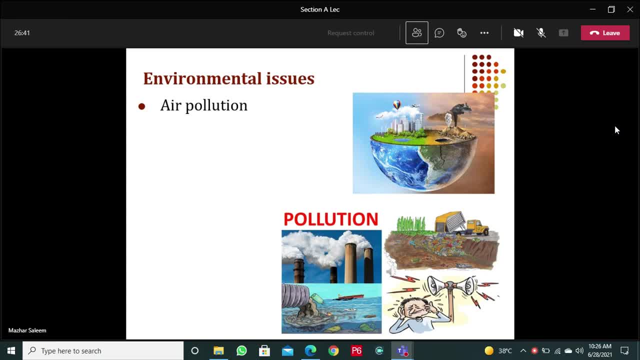 You can add Or you can exhaust the smoke From the chimneys of industry And similarly for the water pollution. There are laws Which tell That how much water pollution can be Or how much Level of pollution can be present. 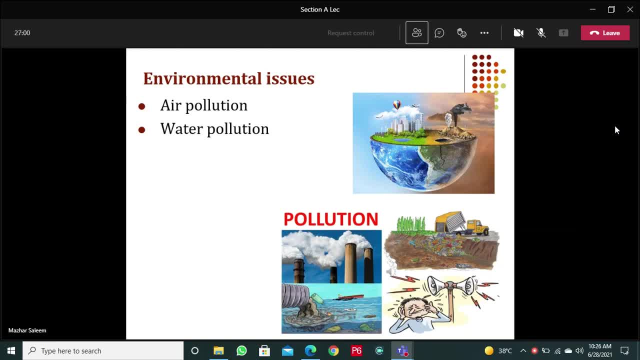 In the wastewater of any industry, And then government Bounds the Industries to Install wastewater treatment plant, So they have to treat their Wastewater before Disposing it off in any water body. And noise pollution, Civil engineering projects. 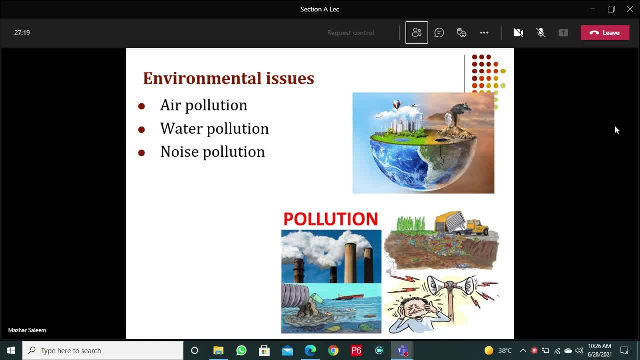 Contribute towards Noise pollution as well. So We need to, We need to take care of that as well. One of the examples is Driven piles. When we install, When we carry out any large scale projects And let us say we are doing piling for that. 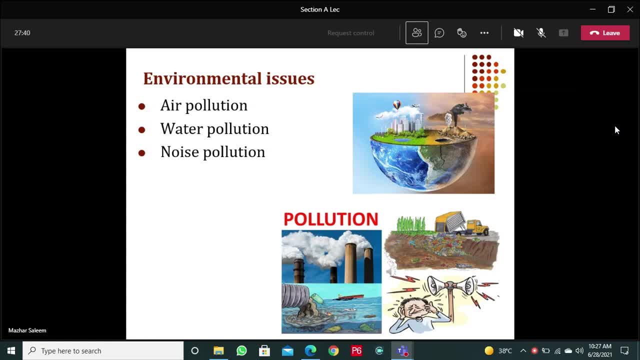 So there are two types of piles. One are drilled piles, For which we drill holes And then cast the piles. Other is the driven piles, Or hammered piles, Which causes significant amount of noise. You can Look for any videos of hammered piles. 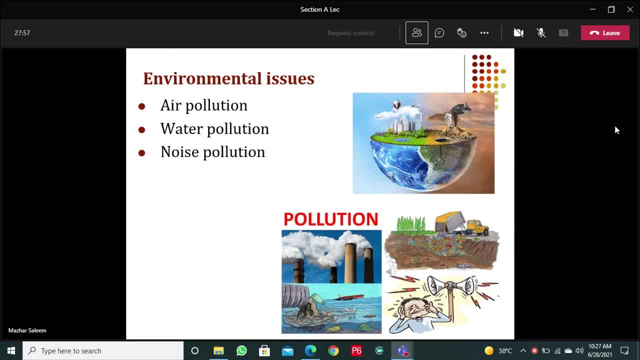 Or driven piles on YouTube, And you will find that when we do hammering, It causes significant amount of noise. So When we execute projects, Depending upon the location of the project, When we are selecting the, The type of pile that we need to install, 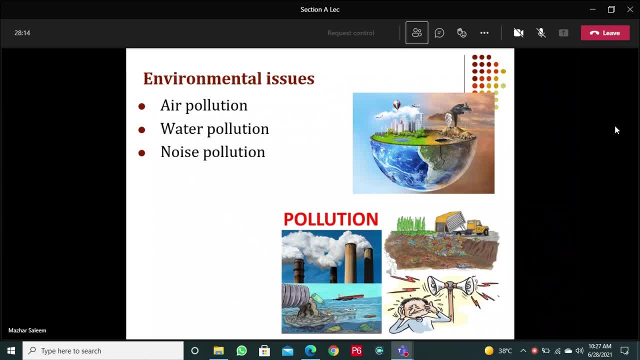 We have to take care of The noise factor as well. And This brings another important thing in our mind: That whenever we execute Any large scale project, At the time of approval of the project We have to present a report, Which is known as. 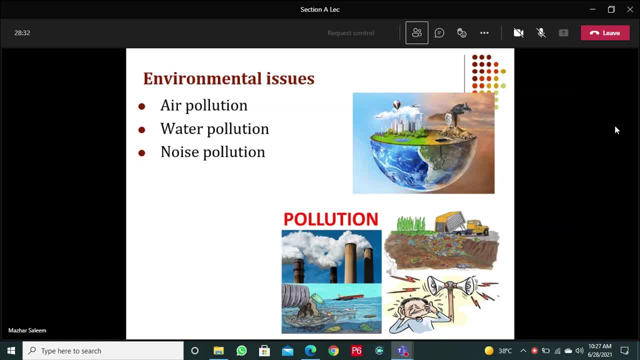 Environmental impact assessment report. So for all the large scale projects We have to carry out a study In which we see that How our project is going to affect the environment. And Currently you guys are in sixth semester In your next year. 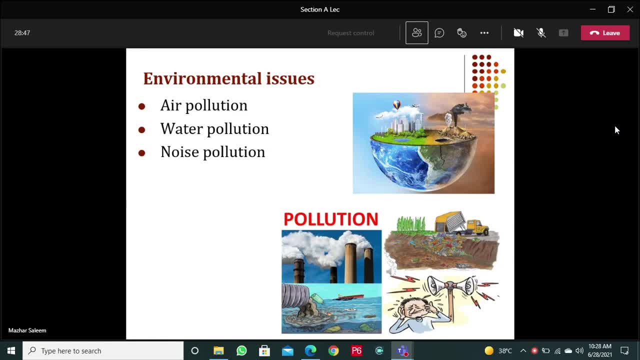 In seventh semester And eighth semester You are going to be in two subjects On environmental engineering: Environmental engineering one And environmental engineering two- And in those subjects You will be taught that How to compile an environmental impact assessment report For any project. 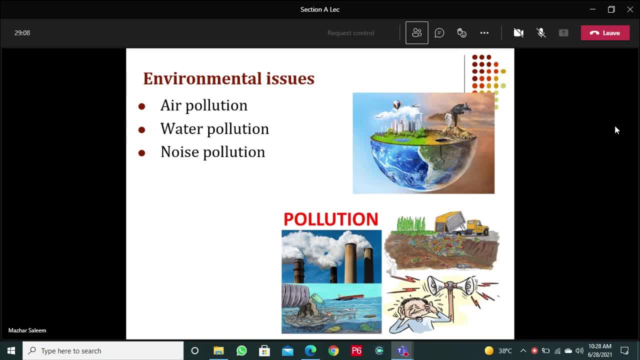 Let's say, If you are working on project of a dam- Now, dam is a huge structure- You obstruct The path of a water body, So you build a huge wall, Either maybe concrete wall, And that Results in the creation of. 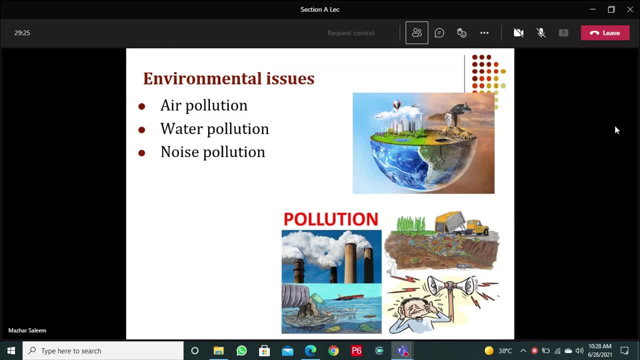 A huge reservoir of water And that changes the entire ecosystem Of the Of that locality. So go area, Which was First outside of the water, Now it gets submerged in the water, So new water species Will be Will develop. 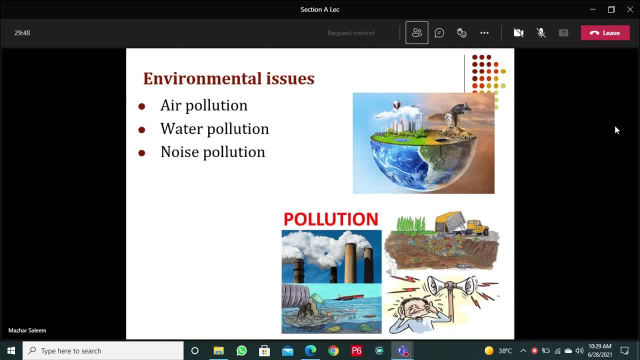 In that area, Or Those birds might Migrate from that location, The plants Will get submerged in the water, The human population Will have to displace, Will have to displace the roads Or other infrastructure, So it will change the entire ecosystem. 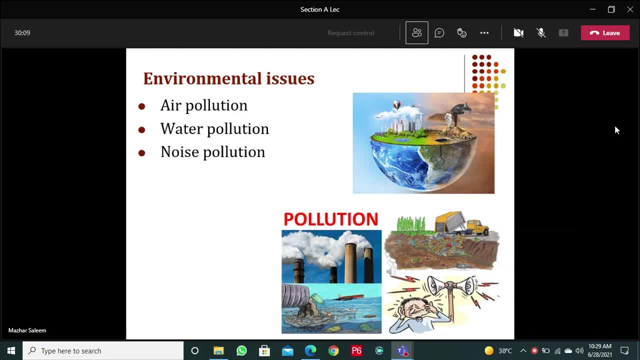 Of that, Of that location. So for such huge projects, And similarly, if we have, Let's say, a highway that runs Over hundreds of kilometers, So for such large projects, We have to carry out Environmental impact assessment report. And in that report, 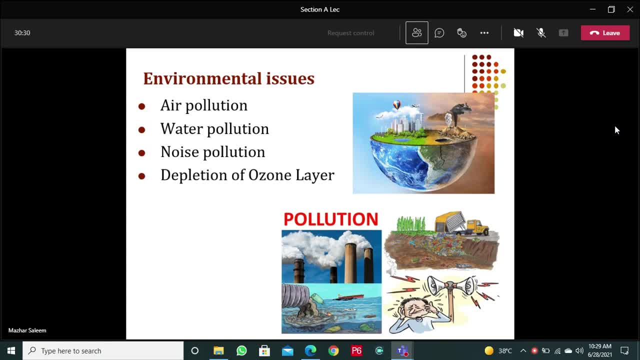 We consider all these factors, Whatever environmental impacts are there: Depletion of ozone layer That's a result of Air pollution. Environmental disasters, Like tsunami, Which is related to The change in the climate. Deforestation: Human beings are. 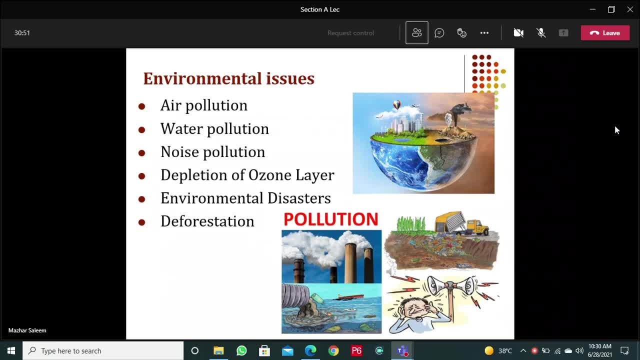 Deforested For housing Societies Or other industry Or other projects, So that deforestation is negatively Affecting the environment. Global bombing- We all hear this word a lot- That because of increased amount of Pollution of carbon dioxide. 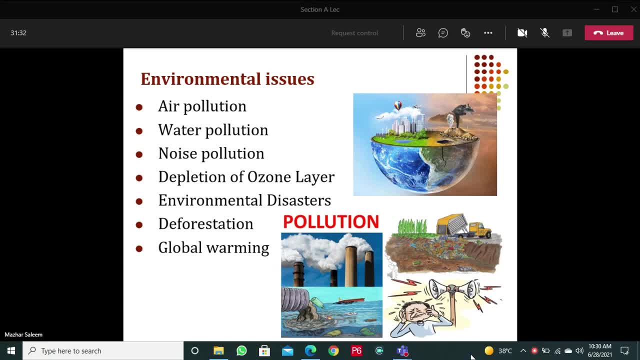 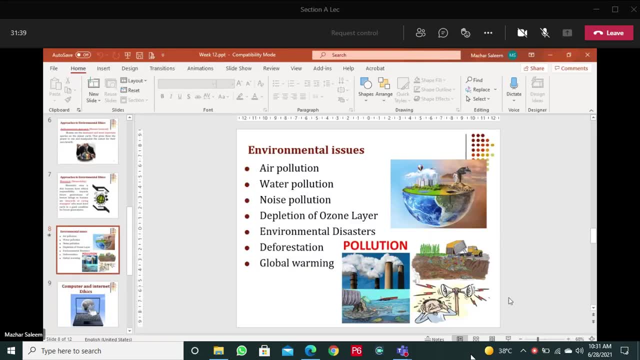 In the environment. The overall temperature of the Earth is increasing And that is causing The climate change. And after this We move to the next topic. So any question about Environmental ethics. guys, I'll wait for a few seconds. 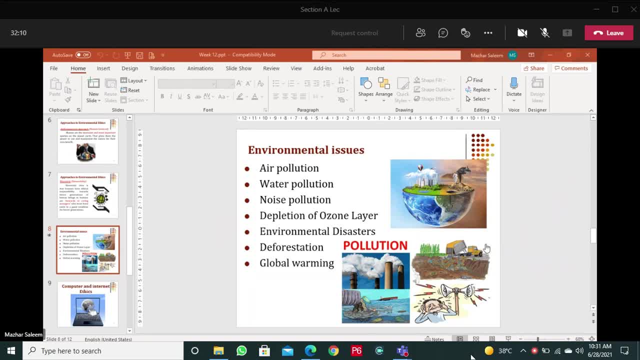 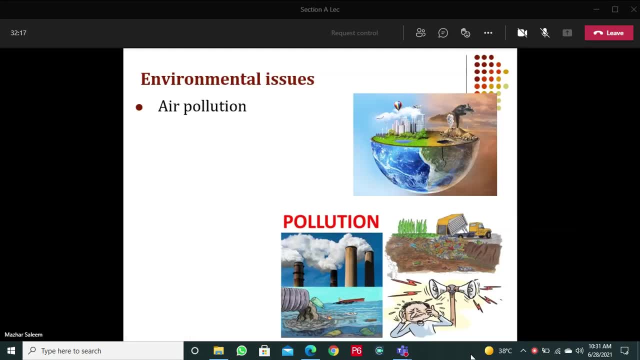 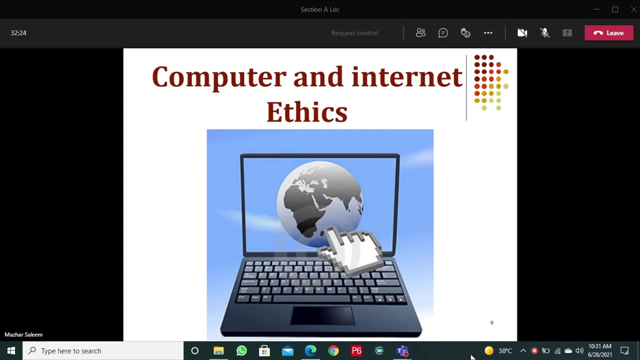 Okay, so If you guys do not have any question, Let's proceed with our discussion. So the next topic, The last topic that we are going to talk about, is Computer and internet Ethics. So before I start explaining this, I would like to hear some. 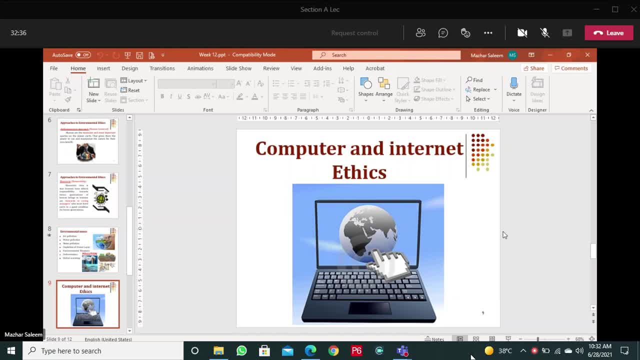 Points from you guys. What do you guys think Are the ethics For the use of computer and internet? And this is. These ethics are not just limited To the use of computer. now, I'm using this term because It's a part of our course content. 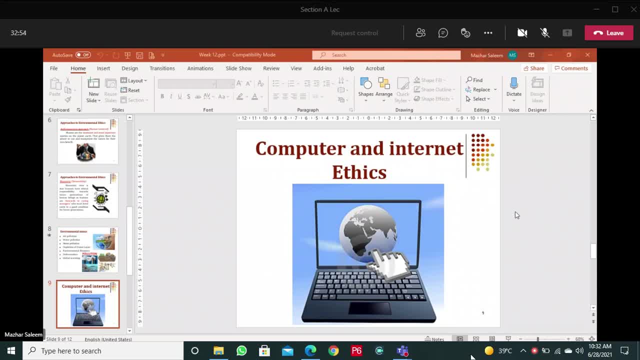 But actually It includes The ethics for All the electronic devices And internet that we use internet on, For example, tablets Or mobile phones Or laptops- Any electronic device. Okay, Would anybody like To comment on this? What do you guys think? 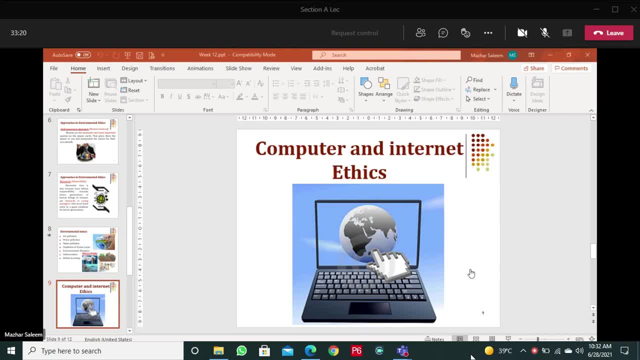 What are the ethics? Jahangir M Jahangir, Are you there? Seems that Jahangir is not there. Bilal, Bilal, are you there? Okay, Bilal, So would you like to comment on this? 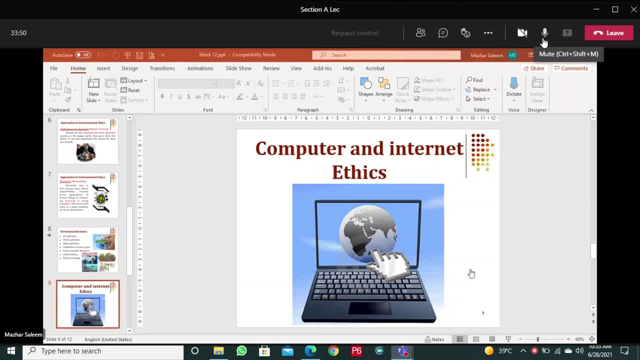 What do you think are the computer ethics, For example? What are the ethics To use in a positive way, To use in a negative way? What can be a negative use Of devices? There are scams. That's true, Absolutely right. 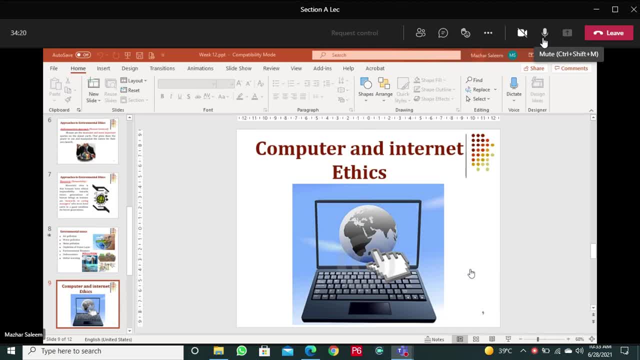 Scam. Scam In financial transactions. Okay, Okay, All right, Anybody else? Rohan Rohan, are you there? Yes, sir, Okay, Rohan So Rahman, What do you think? What are computer ethics Or what are some negative uses of computer? 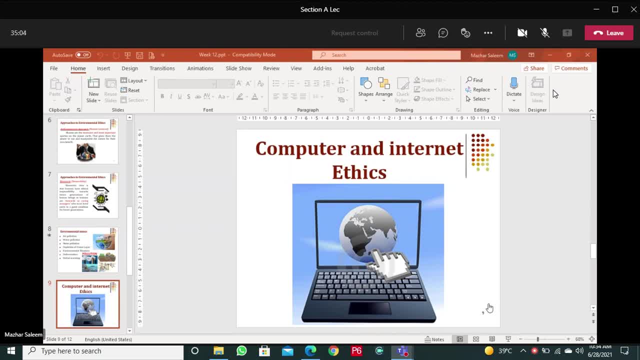 Let's say, If I rephrase my question, It can be related to a company's property Or a company's privacy In computer ethics. Privacy, That's right. Privacy is very important. We need to respect the privacy of others. 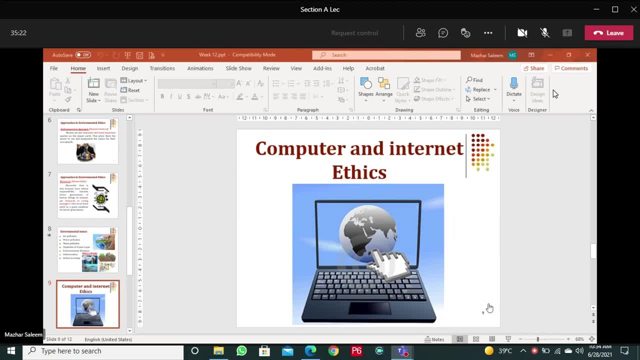 Who are using computer. That's true Computer crime, Cyber crime. Cyber crime. Right Data leak- Last time, Okay, Cyber crime. There is privacy And data leak. Cyber crime, Property record, Software protection. Software protection. 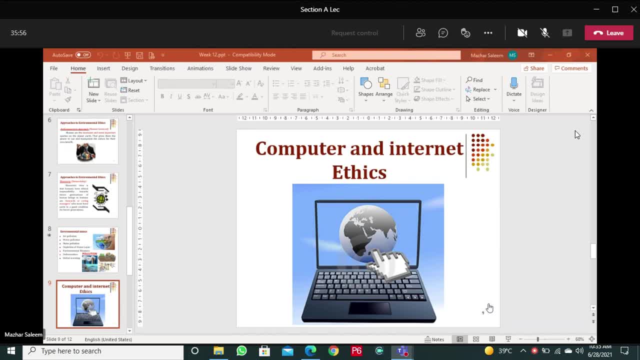 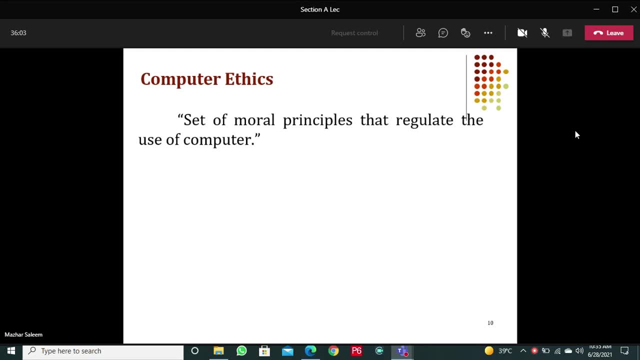 Yes, sir. Okay, All right, Thank you, All right. So let's see. Computer ethics are set of moral principles That regulate the use of computer. These are the principles that tell us How to use computer. And if you do a little, 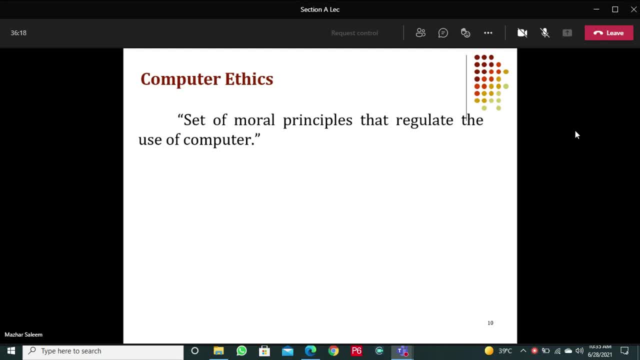 Search on Computer ethics You will find that there are 10 commandments of computer ethics. Those are very popular And a lot of people have reported those commandments. So I have also Tried to Report those 10 rules With slight modification. 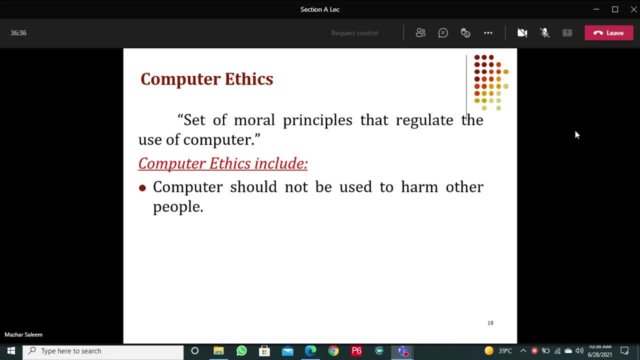 So let's see Computer ethics. First one is: Computer should not be used to harm other people. Now, this is a pretty general, Like general, rule. So whenever you are using computer You need to see that you are not Negatively affecting anybody else. 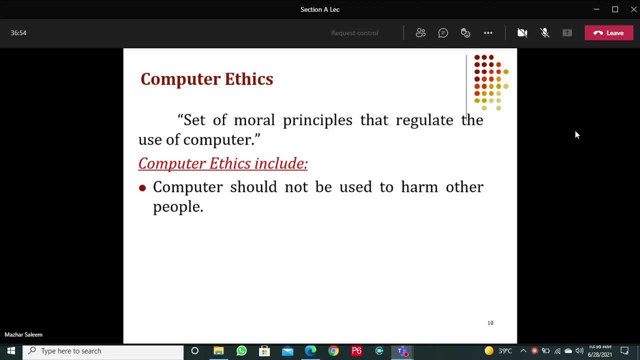 And there are several different ways of Negatively affecting others By the use of computer. You will see those examples Just in a short while, But this one is a Is a general one, But later on, If you are using computer, 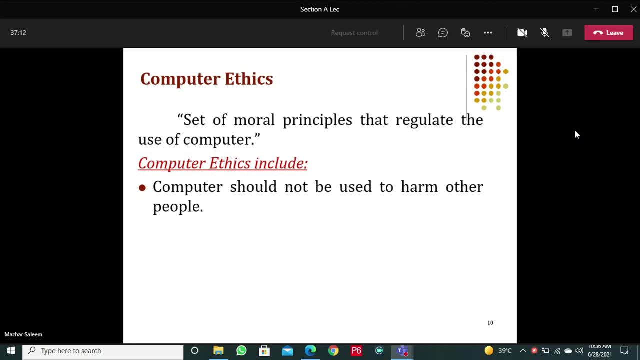 Then, just whenever you are using it, See whether Your activity on the computer Will negatively affect anybody else or not. If the answer is yes, Then that activity is unethical. Okay, And that activity can be of Several different types. We are just going to talk about those types. 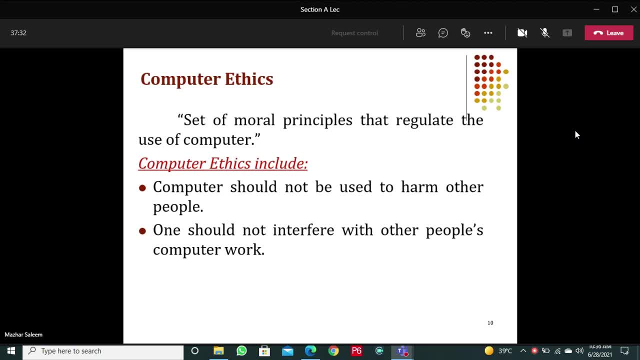 So one should not interfere With other people's computer work. Now, what are different ways Of affecting other people's work? One of the example is Viruses and malwares. So there are people who write Viruses and malwares. 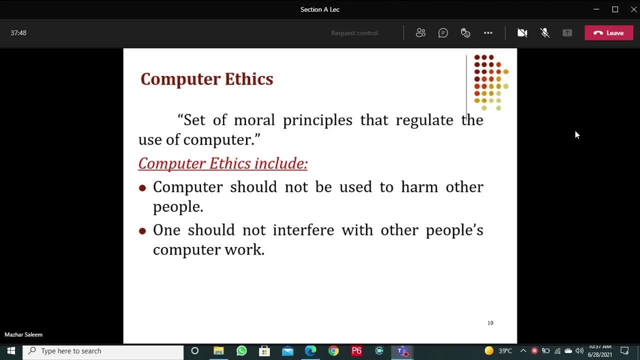 And those viruses can negatively Affect other people's work. People's files are deleted, People's files through malwares. Sensitive information Can be copied And we all have experienced This virus issue, Even if your data is not. 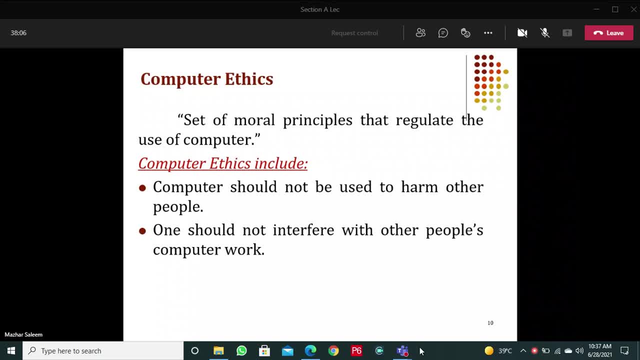 Stealed. It creates a lot of problems for you And several times you have to Reinstall your windows. Whatever software you have installed, You have to reinstall them. You reinstall the windows, So it wastes a lot of time And sometimes some of the useful data. 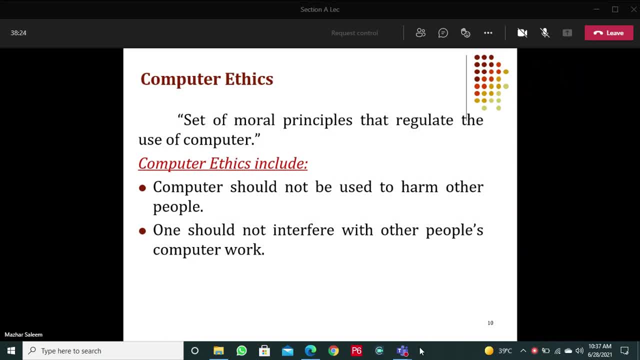 Is also wasted, So the creation of viruses Is an unethical activity. Do not snoop around Other people's files, And this is especially important When we are using public computers, Computer labs. You are working in a computer lab Of the university. 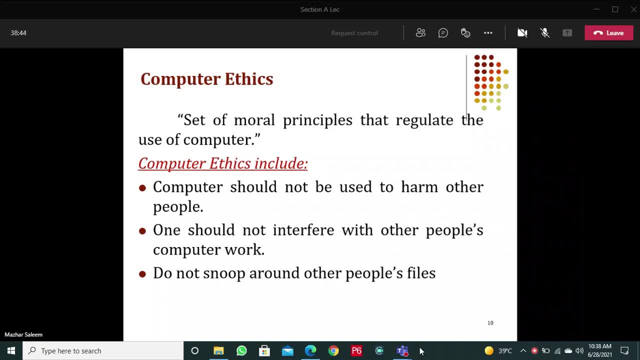 Or later on, when you are working In a professional organization And there are some common computers, Or in a library. There are common computers, So the common computers Can contain other people's data And it is unethical to snoop around. 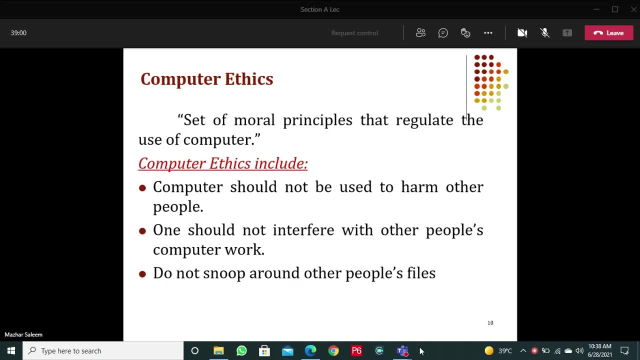 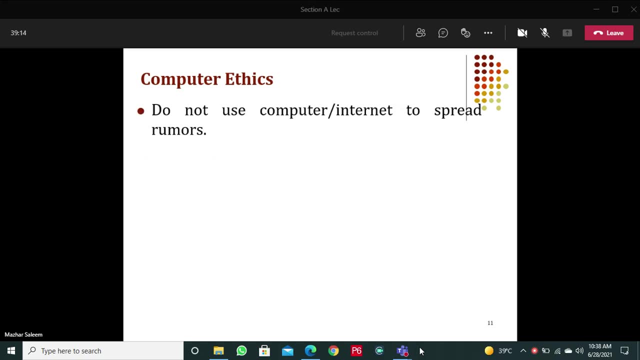 Those files, To dig those files, To see what is in those files. That is an unethical activity. Whenever you use public computer, Just focus on your personal work, Do what you have to do And do not interfere in those files. Do not use computer or internet to spread rumours. 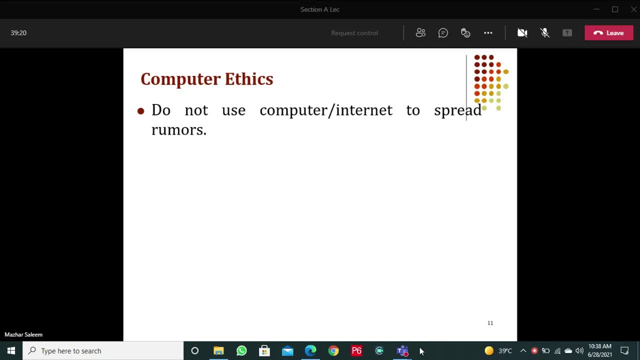 Now, this is In the recent times. Spreading rumours through computers Has become really common. So, as a Responsible professional And as a responsible human being, We should never Spread rumours, And in today's world, Spreading rumours is extremely easy. 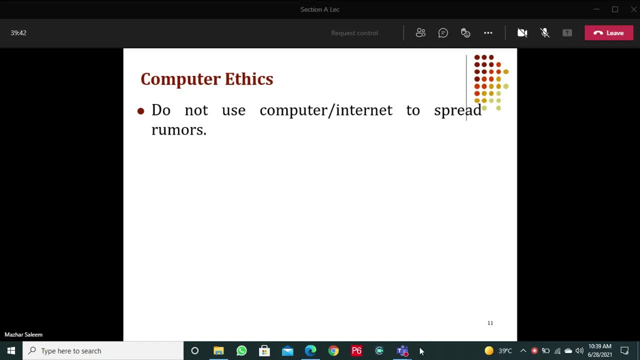 We have a number of WhatsApp groups And Facebook groups And we have friends on Instagram. It is very easy to spread any rumour, But spreading that Is totally unethical. We should never share anything Or any information, Any post, that we are not sure about. 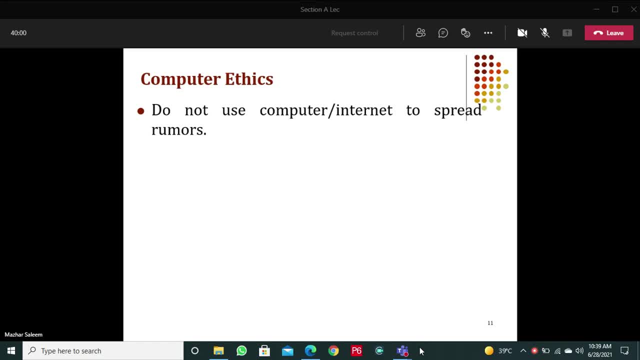 If we are doubtful about this information, We do not have authentic information On any topic. We should never spread that information. That is unethical. Do not use pirated softwares. Now, this is something Which is unfortunately very common In our part of the world. 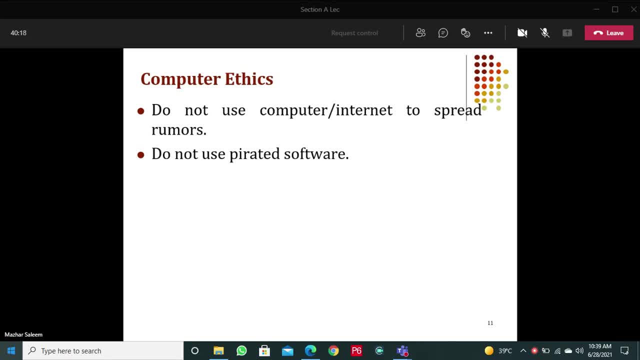 We use pirated softwares, But that is illegal And unethical In internationally. The laws are strict about that. If anybody is found guilty Of using pirated softwares, Then he has to pay Heavy damages And fines for that. 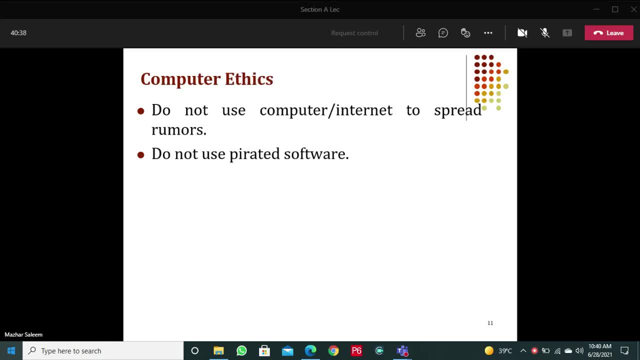 Unfortunately, The rules are not that strict In our part of the world, Because probably we cannot afford all these softwares. That is why piracy is common. But we need to know that this is wrong And if you ever Get a chance to work abroad, 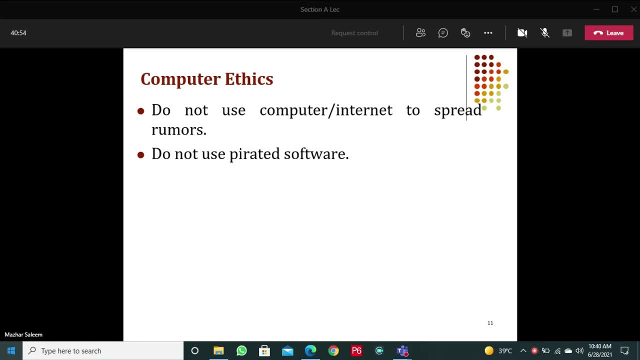 You need to be very careful about that, Because there Abroad This is not just unethical, It is illegal And people are strict against piracy. Do not use Other computer resources Without authorization. Now, what does this mean In organizations? 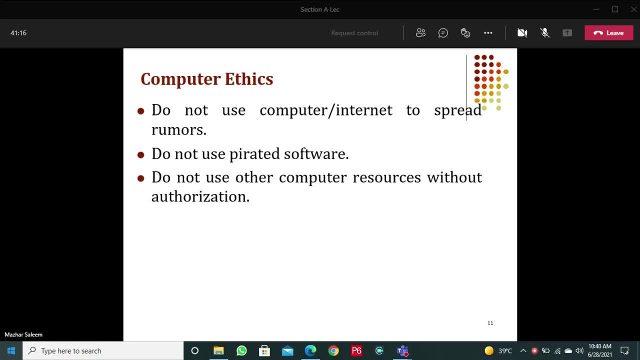 In professional organizations, Every person has a login. For example, Even in our university Logins, Teachers have their own logins, Students have their own logins And different logins have different levels of access. Take, for example, Student ID. 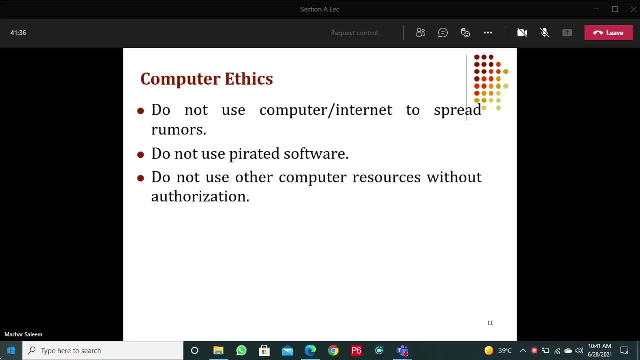 And your student login Can help you to see your own DMC. Let's say, As a teacher I can see DMC of all the students, But I cannot edit that, But some other person Who is an administrator of, Let's say, LMS. 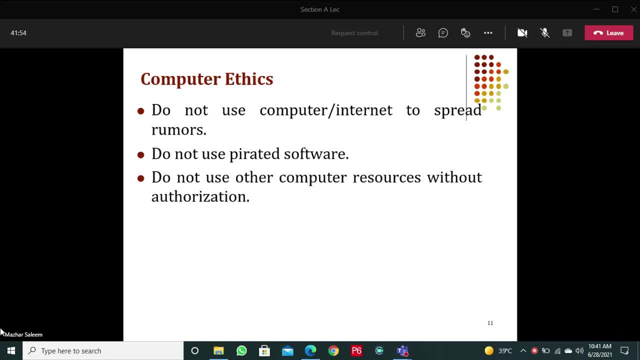 Or controller of examination. He can see the DMC of all the students And further He can make alteration in that as well. Right In an organization. Sometimes, when you are working in an organization, What you see is That a person was using a computer. 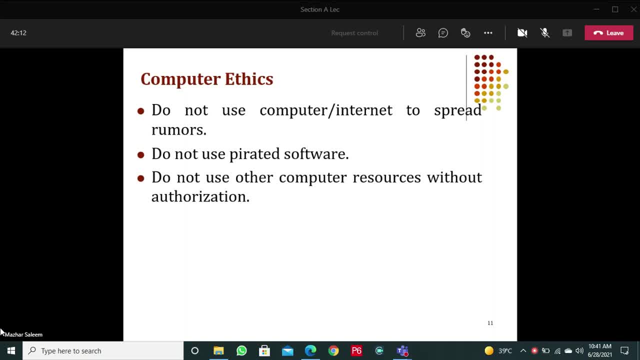 And then he left And he forgot to log out From his account. And then you get an opportunity To use his login. But using his login is unethical. If you have access to that login, If you use that access, Even if it is not a different level of access. 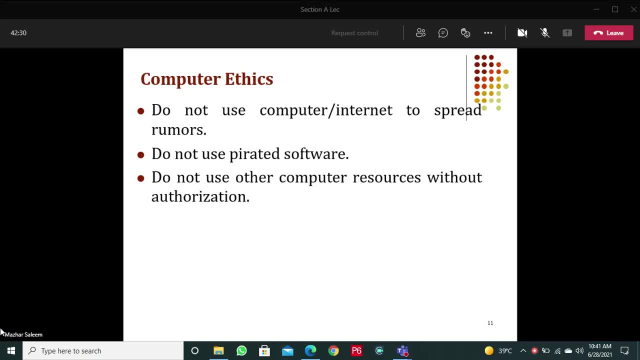 But your friend's login Or your colleague's login And you use that And you do any activity That you are not supposed to do. That is an unethical thing to do. If you ever get a login, You must log that out. 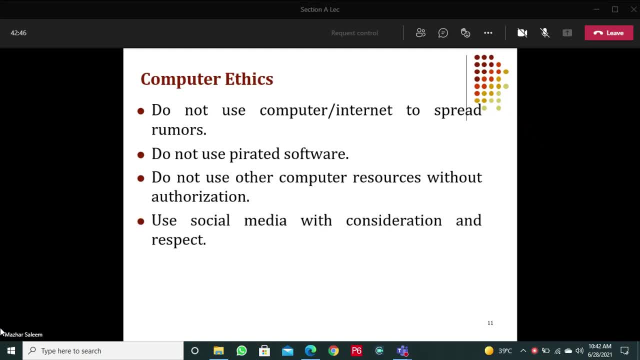 Immediately Use social media with consideration And respect. Now, this is another problem of our time: That in social media We see that a lot of people Bully others. They are very rude, They post harsh comments On others. That is not a good thing to do. 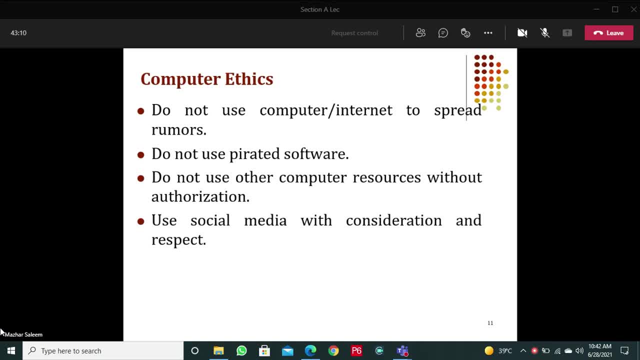 If you disagree with somebody, It does not mean That you start abusing Or harassing that person. If you disagree, You can show your disagreement. That is totally fine. But whatever you say, You are supposed to be respectful And considerate towards others. 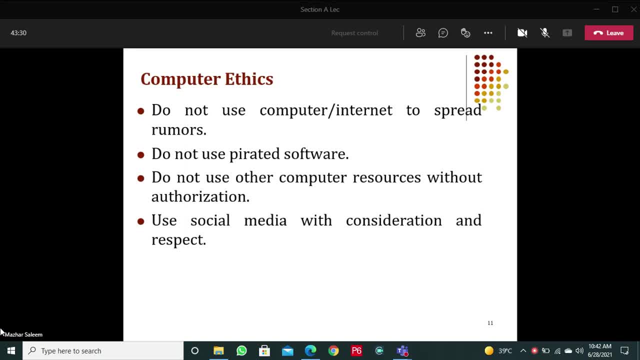 And when we Like. few weeks ago, We were talking about Disagreement, or the points That we need to keep in our mind By criticizing others. So you need to keep all those points In your mind By using the social media. 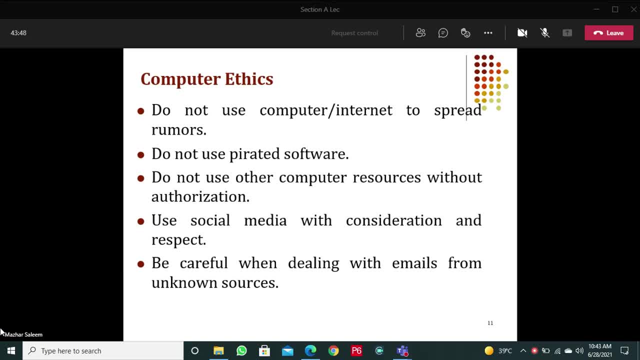 Be careful when dealing with Emails from unknown sources, So this is something which is Important for your own safety. A lot of times we get emails Which are basically scams, As some of our friend also mentioned that There are a lot of scams on internet. 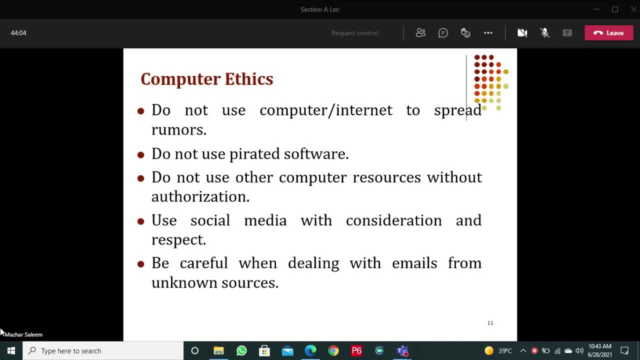 So if you ask us to open an attachment Or click on a link Or reply with certain email, Reply with certain information, All such emails are Scam emails or phishing emails, So we should be very careful While dealing with such email. 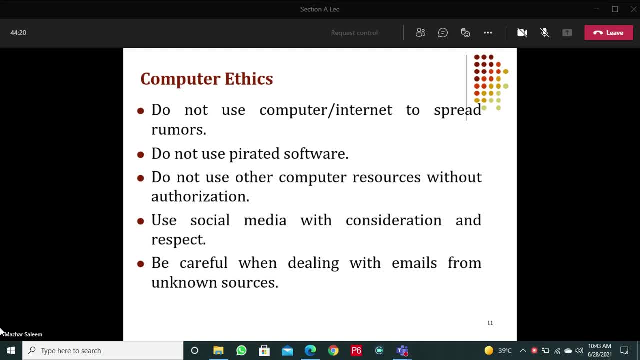 If you are getting an idea By looking at the subject of the email, That is something not relevant to you, Don't open such email. If you have opened that email, Read it carefully If you think That it is a scam. 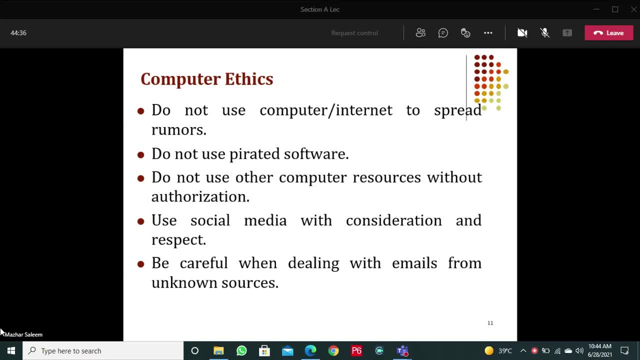 Do not click on any link And there is an easy way To identify these scams. A lot of times There is no proper signature. People don't show their name Or designation in detail Website Or from which organization they belong. 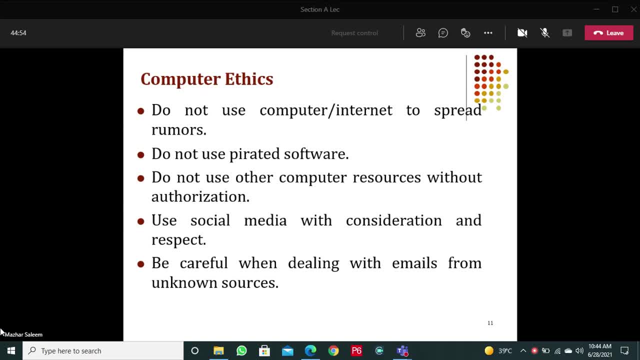 There is vague information. Sometimes People will pretend That it is an email from a university administration, But under that There will be only a name, No proper designation. So these are some of the hints Or clues That help you in identifying. 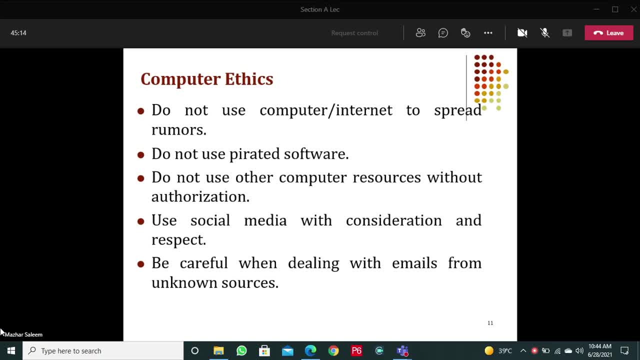 That whether an information Is valid, Whether an email is a genuine email or not, And one precaution that you may take Is that if you are in doubt In some of the cases, Then whatever, From whatever organization That email appears. 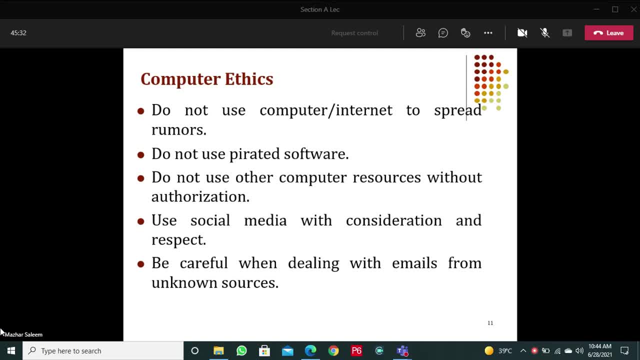 To be. You can send a separate email To that organization To verify that information. Sometimes you will get an email Where they will offer you a job And people get excited about that, Especially at the beginning of the career, If there is an email. 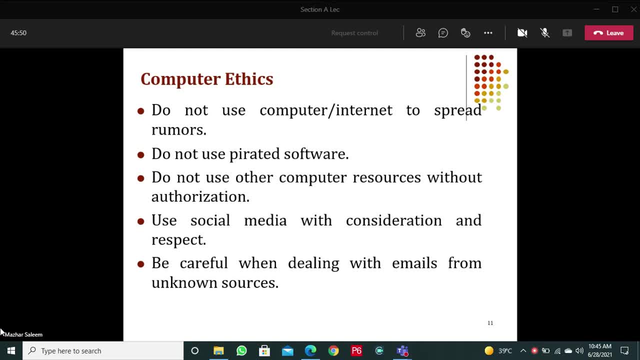 Like you are already looking for a job And you find an email In which you have a job offer, Then that might excite you And in that excitement You might respond to that email. So if you are in a situation Where you think 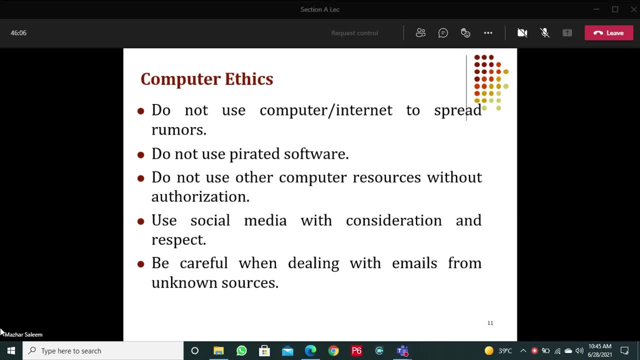 That it might be an important email And you might miss something If you don't respond to it. So the best way is That you write down a separate email To that organization And you verify that. Is it true, Is it valid or not? 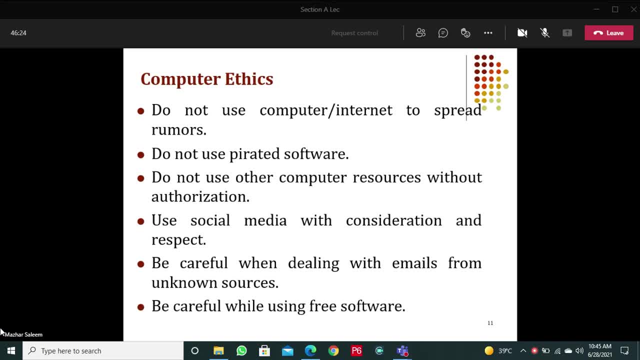 So these were Some of the ethics That we need to keep in our mind While using The internet. The last one is: Be careful while using free softwares. So these free softwares, Or pirated softwares, These softwares are also a source of viruses. 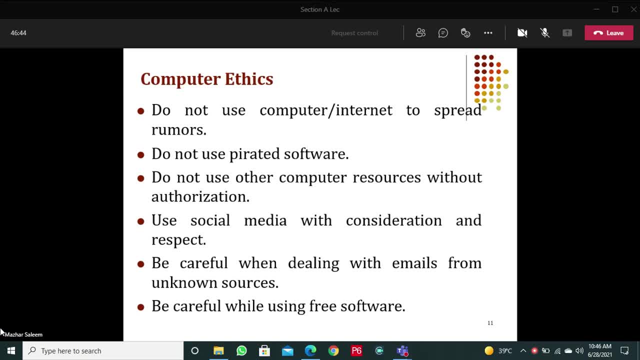 You see, Because a lot of times We are looking for free softwares. So that search sometimes Takes us to some websites Which are unsafe, And when you install software And download it, Malwares can get into your system, And sometimes they do. 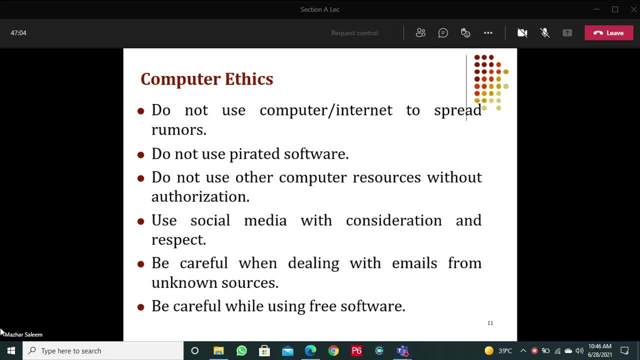 So, whenever we are using Free or pirated softwares, We have to be very careful. Okay, So these were some of the ethics That we need to keep in our mind While using the computers. But this, The discussion about this. 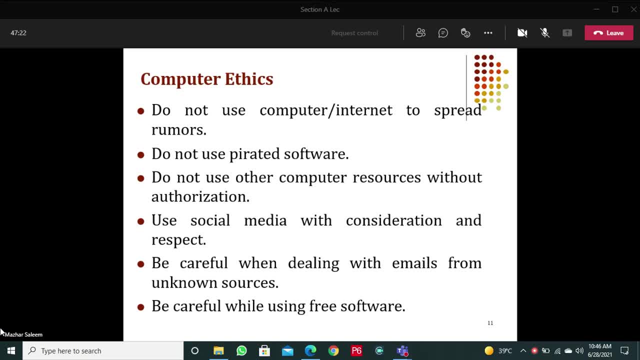 Computer ethics. The formal discussion is over, But there are a couple of manners as well That I want to share with you guys, That you keep in your mind While, While dealing with computers, Sometimes we visit somebody else's office. Let's say, you go to your teacher's office. 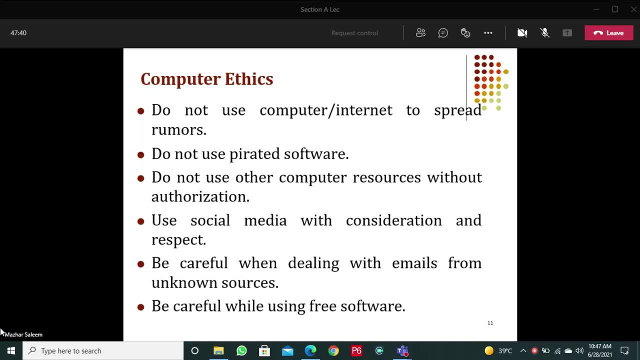 Or your boss's office. So one manner is that You should not stare at the computer screen. If there is a computer there, If it is facing towards you, Do not look at that screen. And if there are multiple chairs available In the room. 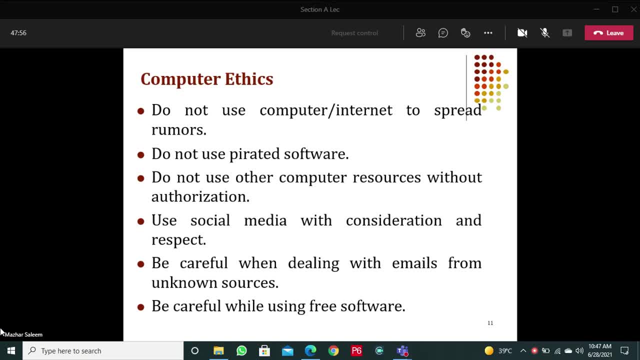 Then try to place yourself in a way That you are not facing the computer screen, Because the computer screen is inclined. If you are sitting in a certain chair, Then you are facing the computer screen, But if you sit on some other chair, 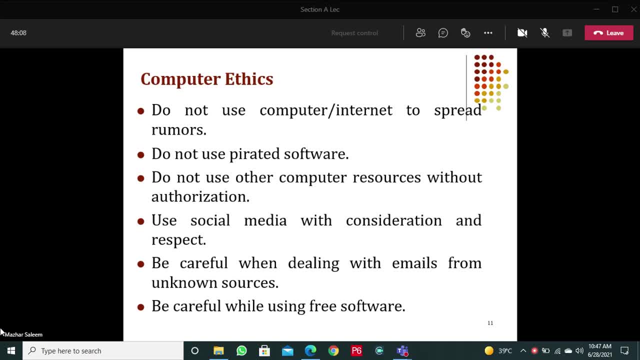 Then you will not be facing the computer screen. So one manner is That you place yourself in a way That you are not facing the computer screen So that you cannot see That what other person is doing on the computer. Similarly, Another manner is: 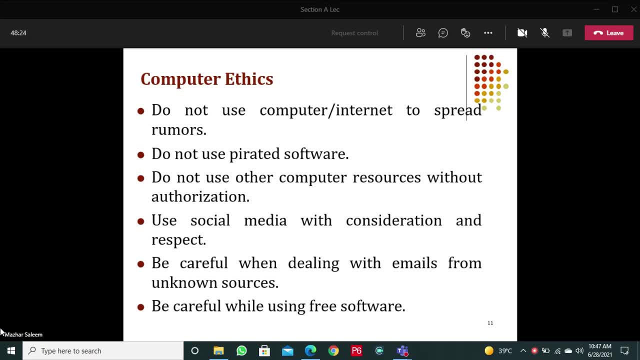 If somebody is logging in Into his or her account, Then you are not supposed to look at the keyboard. If you are a teacher Or your boss And he is logging in to his account, So when he is providing the login information, 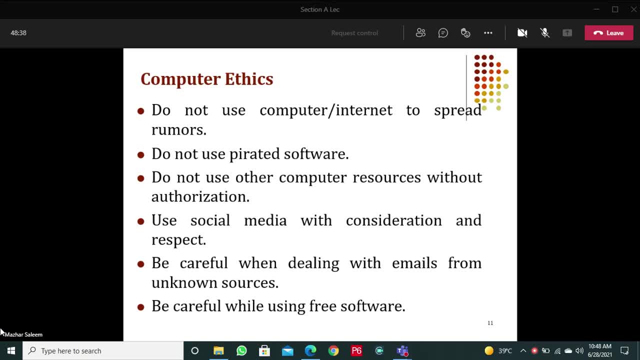 You are not supposed to stare On the computer. Neither you will look at the screen Nor you will look at the keyboard. A lot of times people are not careful in this, But in our country We do not teach this mannerism. 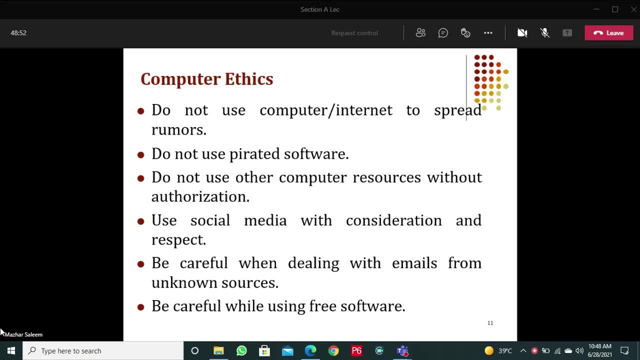 To our students or children. That is why they do not know that. But in the outside world Clearly they turn away their face From the computer or from the keyboard When they see that somebody else is logging in. So it is not like. 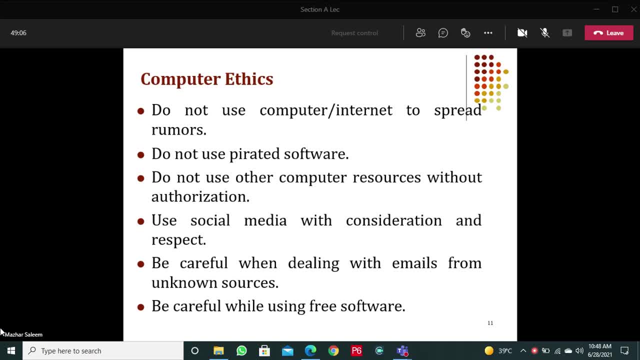 That they are just pretending. They clearly turn their face to the other side So that the other person Can conveniently type in his personal information. So I would like you guys To practice the same thing, That at least When someone is logging in. 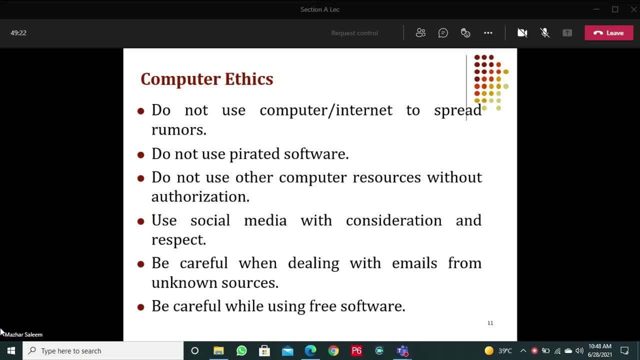 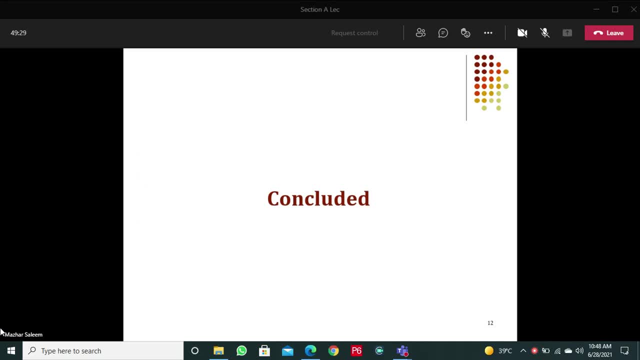 You should not look at the computer screen. That is a basic manner. Okay, So with this Our discussion about the computer ethics is concluded, And this also concludes Our discussion about this course of Professional ethics. We, I think we have. 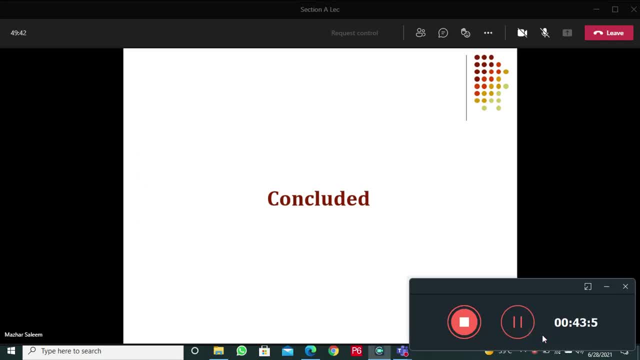 Discussed all the topics In quite a bit detail, And Today was our last week Of discussion about this. Now, Before I used to Ask for questions, I would like to give some concluding remarks On this course That 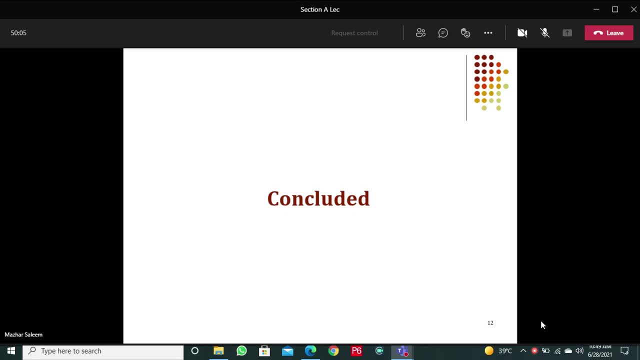 This was the very first time This course was taught In our department And I also taught this course For the first time And I found this course Interesting And I had a good experience teaching This course. You guys are good students. 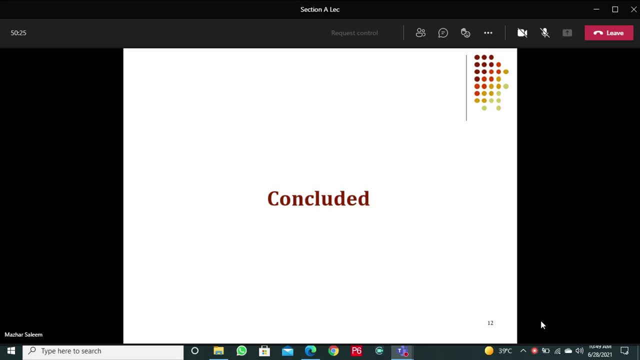 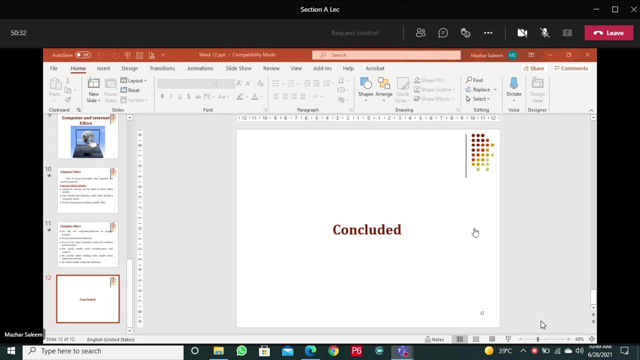 You guys submitted your assignments And appeared in the classes. So we have discussed. Now let me get out of the PowerPoint And come to the screen. We have discussed several different topics In this course, But personally The most, The topic that I liked the most. 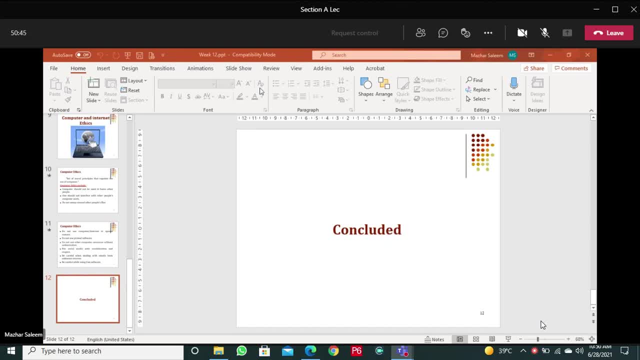 Or that I enjoyed the most Was about self-realization. I think Self-realization That was a very powerful topic, And in civil engineering A lot of times We talk about How to solve any problem, How to analyze a beam. 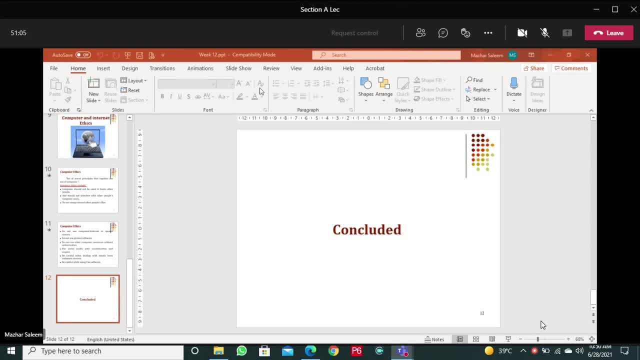 Or a bridge, Or a dam Or a barrage. We just talk about those things All the time And we do not pay much attention To this, This kind of stuff, The topic of self-realization, And I found that 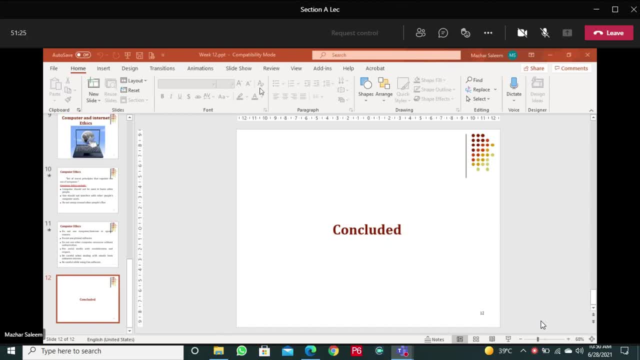 This topic of self-realization Is very profound And more important In any topic That you will study in civil engineering, Because self-realization, It deals with your life And definitely Civil engineering is not the only thing That we will be practicing in our life. 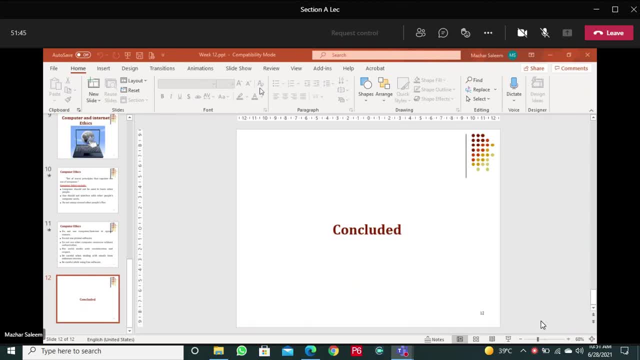 We have several different roles. We are a family member, We are a member of this society, We are a national of this country. We are a human being And we have several different roles As a human being. We have kids, We have siblings. 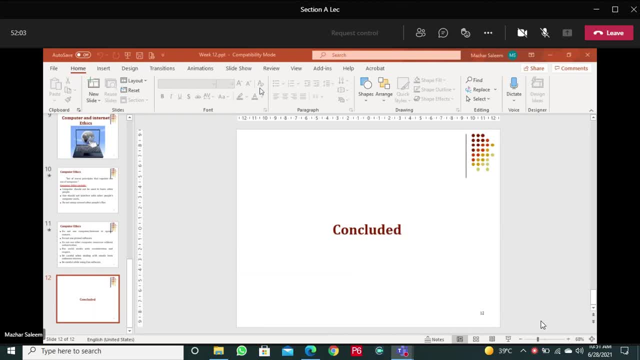 We have colleagues, We have class fellows, We have neighbors. So we have so many different roles And we have our own personalities. We have our own strengths and weaknesses. So the topics that we covered Or the points that we discussed When we were talking about self-realization- 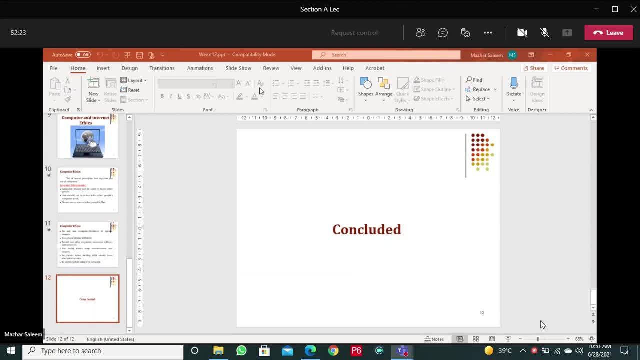 I personally found those points very important. So what I want is I want all of you guys To really work on that, All the topics that we study In civil engineering. There is a limitation of those topics, For example, Those of you. 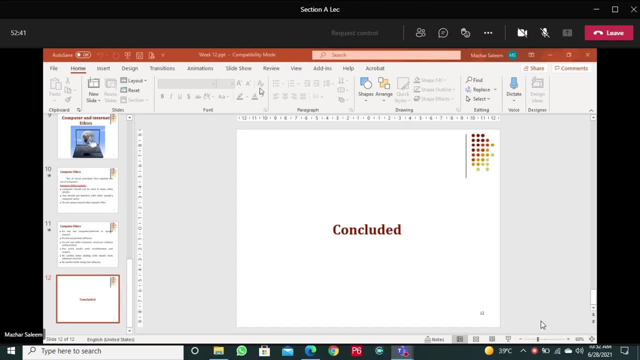 Who will go towards structural engineering: Maybe they will never do Any barrage design Or hydraulic design of a vehicle. They will never do that. Or those who are going into structural design, They will probably never do the survey work Right. Those who are professionals. 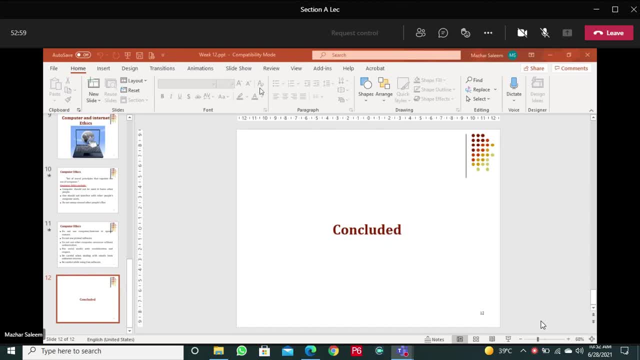 They will never do manual drawing Or you will be using AutoCAD. Those who will go towards geotech: They will never do Structural design of a bridge Or structural design of a building. So when you graduate, You guys will go into different fields. 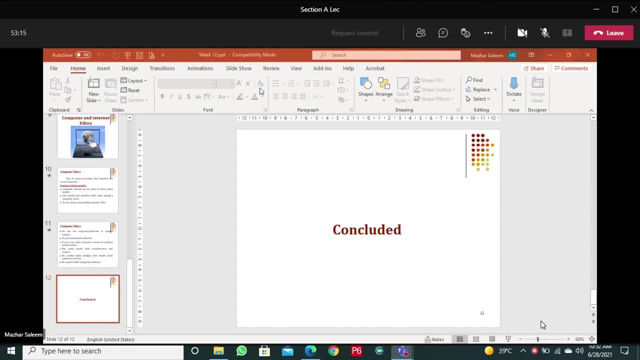 And you guys will have different Areas of expertise, But the topics that we have studied here, The topics that we have studied In self-realization And self-interest, No matter what are you doing, What will you do in your professional life? 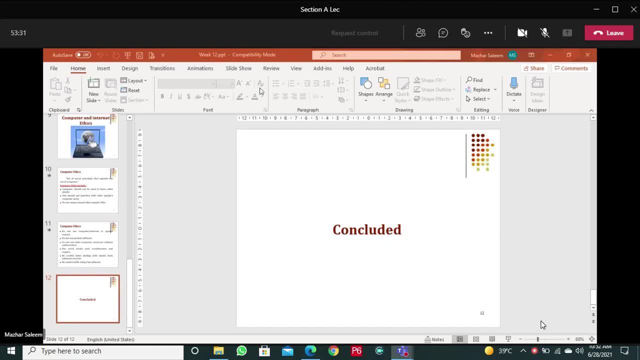 Those topics will always be relevant to you. So, in those topics, The things that we have studied, I really want you guys To practice those things, To practice meditation, To carefully identify your self-interest, Design your life Like you design your goals. 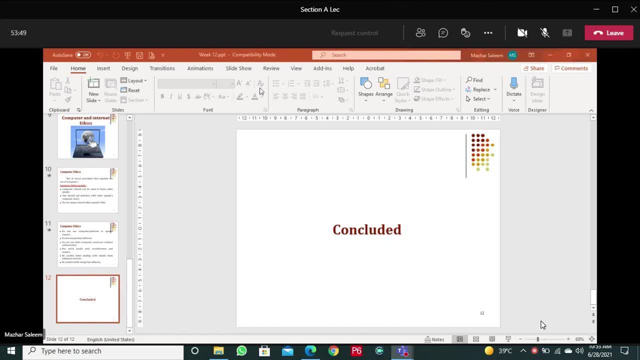 Design smart goals And one offer That I want to give to all of you: That when you are Analyzing your life. I understand that this is very challenging And you will. If you have not done that before, You will find it hard. 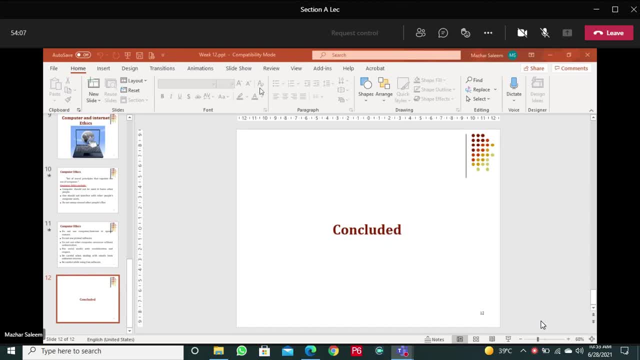 So I offer my personal help to all of you. If you face any difficulty Or any challenge While analyzing and designing your life, While analyzing your personality Or while defining your goals, You can come to me And we can talk about that. 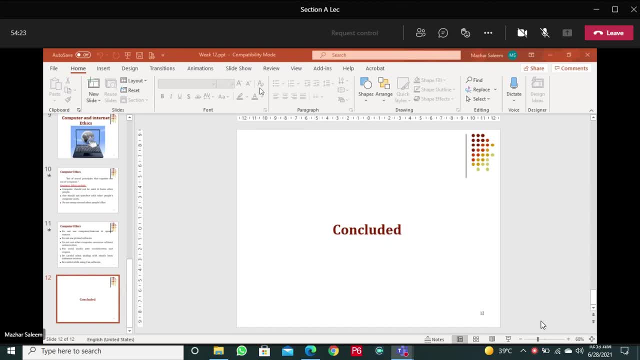 I don't have solution to every problem, But at least I can give you a second opinion And I think I can be helpful In some extent, Because I really All of you are my students And I really want you guys. 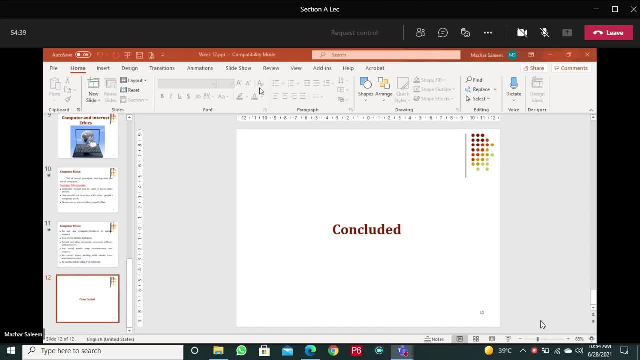 To be successful in your life. So whatever help you need In defining your goals Or in achieving this objective Of self-realization, You can come to me And we can talk about that, And this self-realization Is basically a lifelong process. 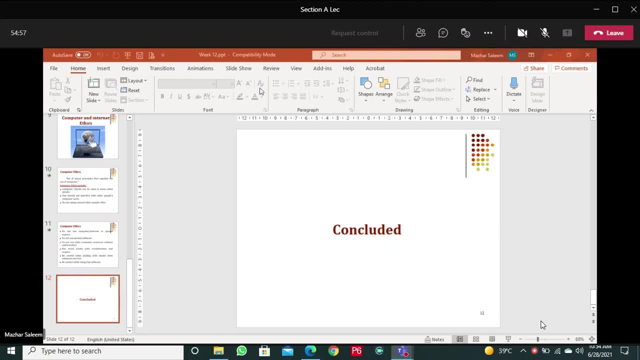 You might not get it even One month or one year. It's a continuous process. You keep on refining it, Keep on refining it And, for the passage of time, You will get a refined model of yourself. Okay, And one last thing regarding the goals. 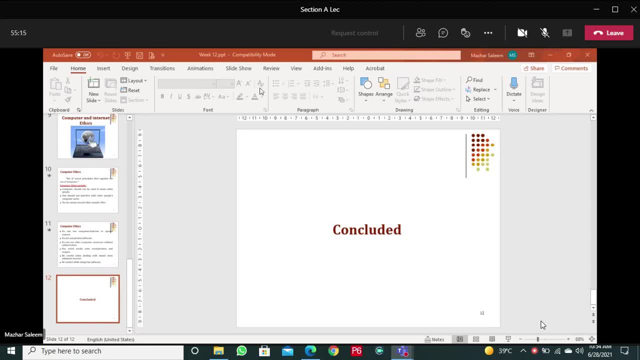 That I want to mention Is sometimes We define goals When we are not able to achieve them. It frustrates us. One way out, As I mentioned before When we were talking about the goals, Was to redefine your goals And keep on working on them. 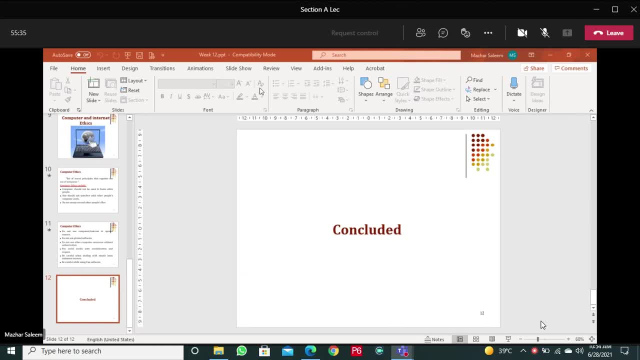 And there is another way, Another way That you will find in the literature, That instead of defining goals You define a process. You say, Let's say, I define a certain GPA, So probably Achieving that GPA is difficult. 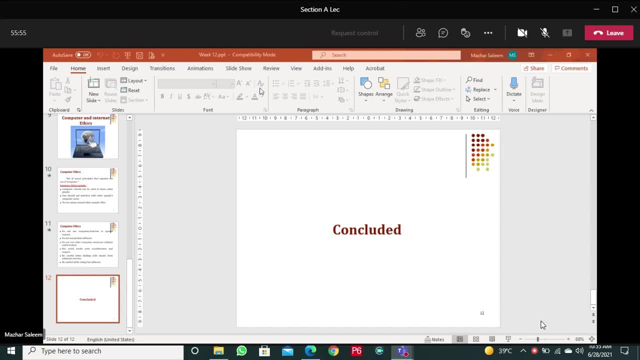 And it's a continuous burden Because you are stressed Because of that. So, instead of defining a goal, You define a process. That process can be Every day. I will be studying, Let's say, for four hours. That's your. 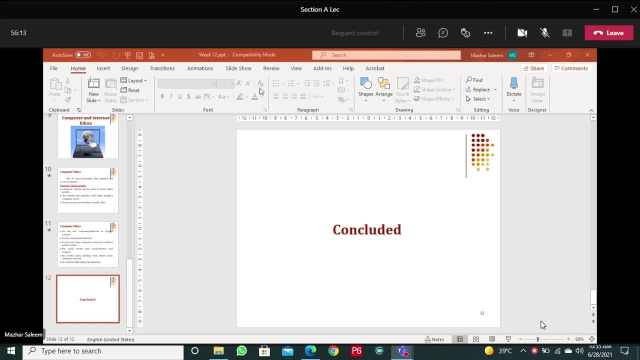 That's a process that you have defined, No matter whatever the outcomes. I will be studying for four hours every day And I will keep on doing it For the entire semester And let's see what do I achieve at the end. And then I refine my process again. 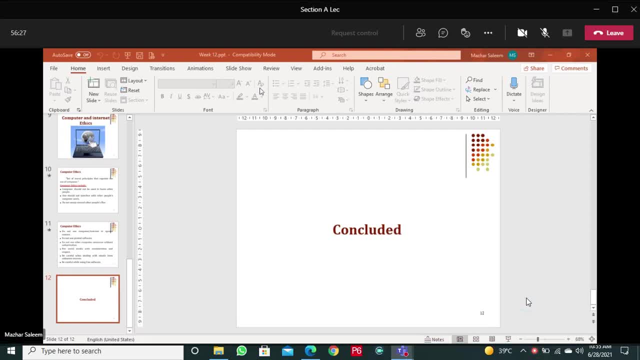 So these are the two approaches That you can use, And with this I think we are running out of time. Let me quickly mark your attendance And meanwhile, If you guys have any questions, You can just leave them in the comments. 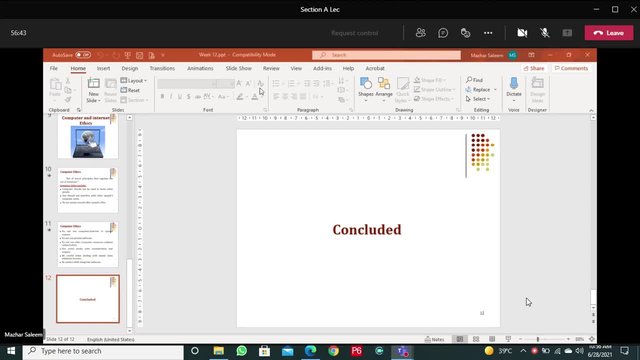 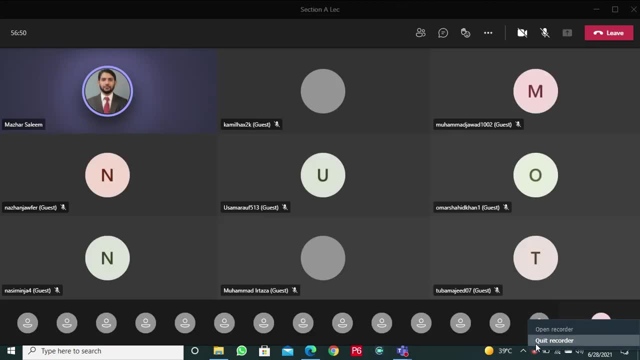 And I will see you in the next video. Bye, Bye, Bye, Bye Bye. you will be asked about the solution, the ethical solution. what will you do in that question? okay, okay, sir. if you are opting a certain option, then why you are?